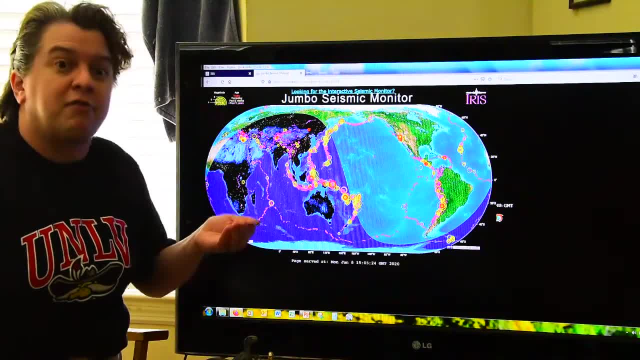 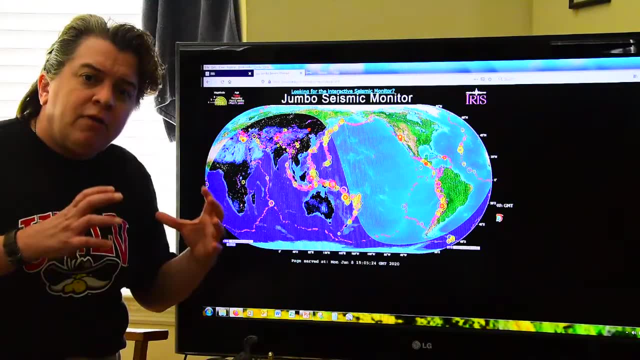 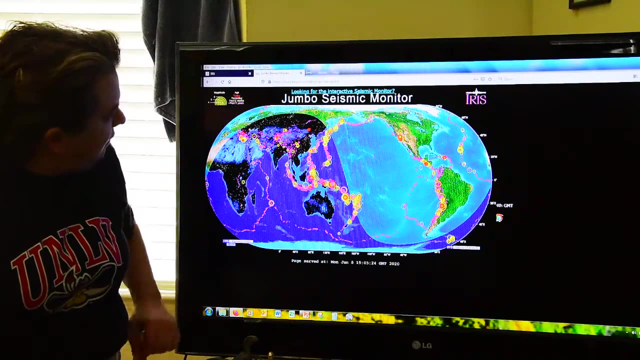 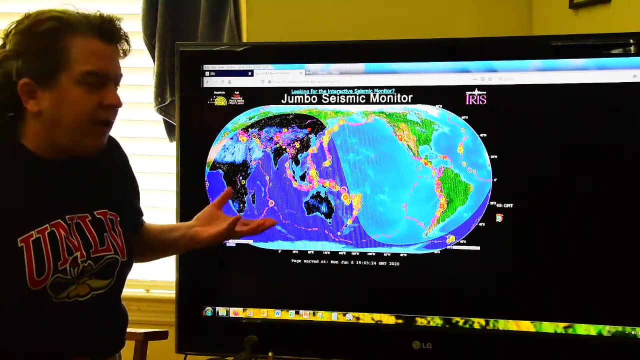 in orange are ones that happened yesterday, basically the last 48 hours, the last two weeks, are shown in yellow and the bigger the circle, the stronger the earthquake was, and this is for me. this is kind of interesting, because there's not any huge earthquakes that I can see, but this is kind of typical, not really that much. 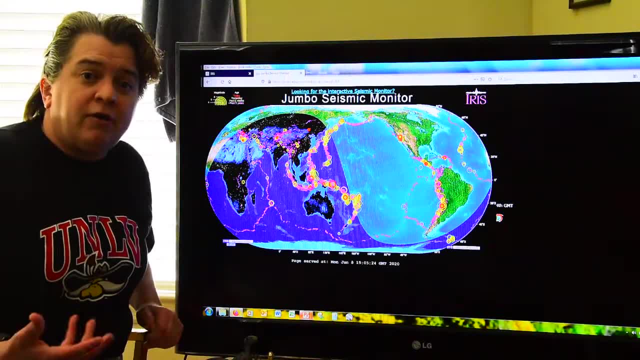 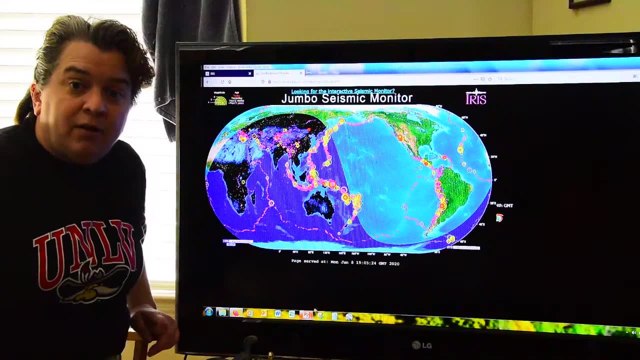 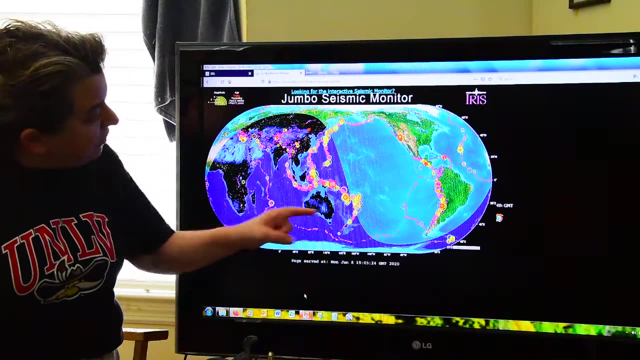 more or less than normal and, like I said, if you're ever curious about earthquakes, go to that website and you can see where they've happened in the last two weeks. so anyway, one thing I do also want to point out is notice how the earthquakes happen in very specific areas. 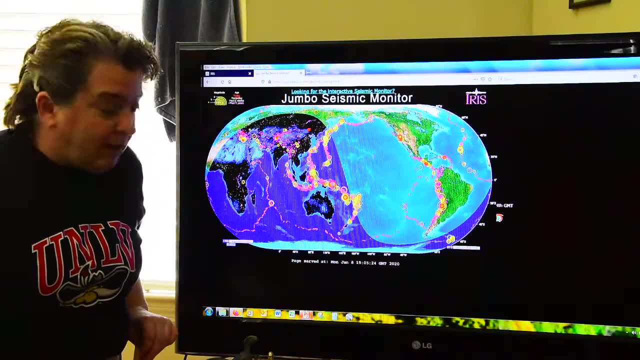 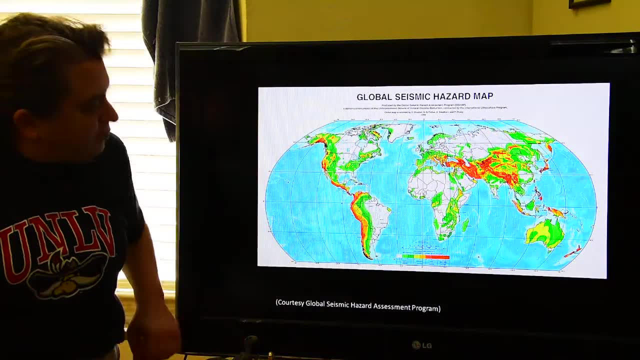 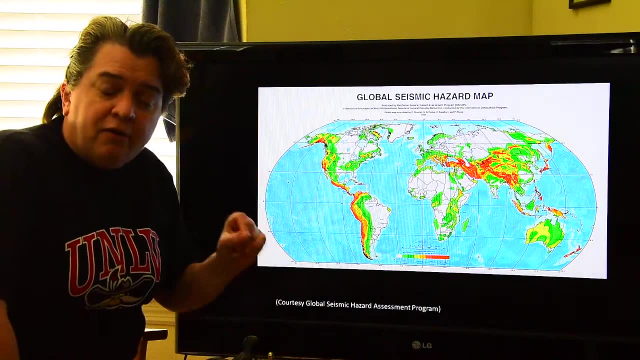 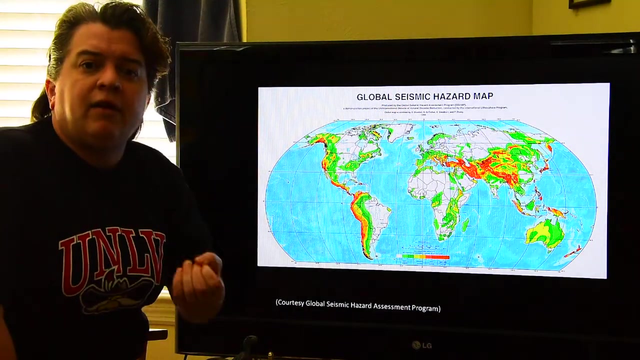 and let's take a look at why that is all right. so here's our seismic hazard map. in red are places that are going to be a higher seismic hazard or earthquake hazard anytime. you see the word seismic, that is related to earthquakes. the greek root word seismos means to shake. 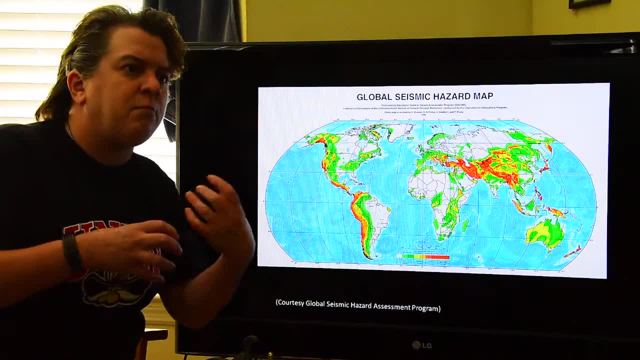 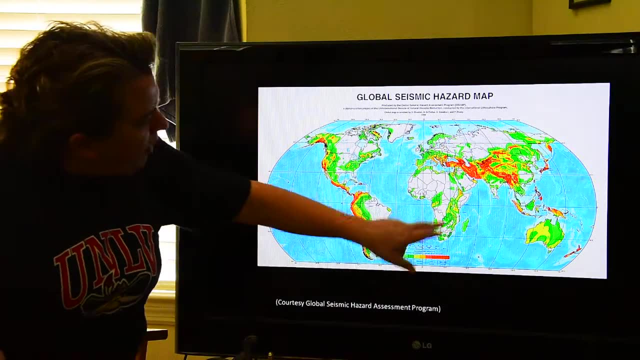 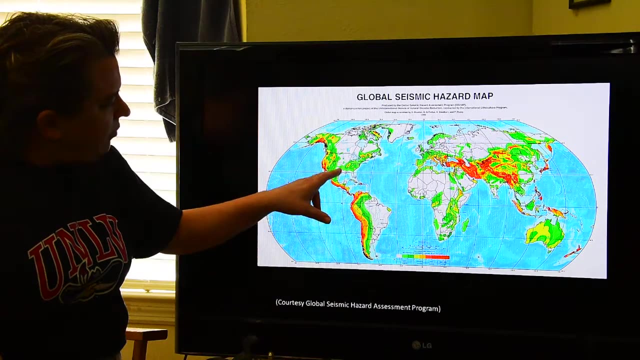 and so seismic, seismogram, seismometer, seismologist- all of those are related to earthquakes, right to the shaking, and so in red we see places that have the highest earthquake hazard, and it decreases all the way over here to white, and I'm not going to say that an earthquake will. 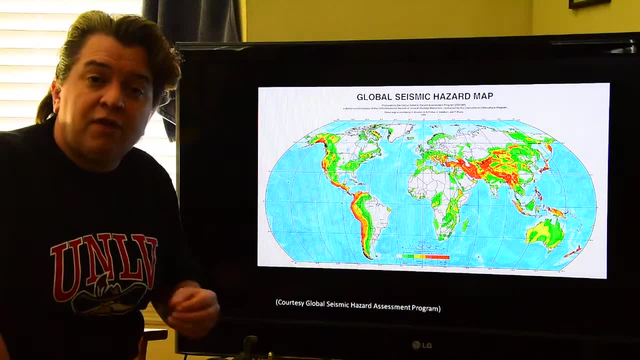 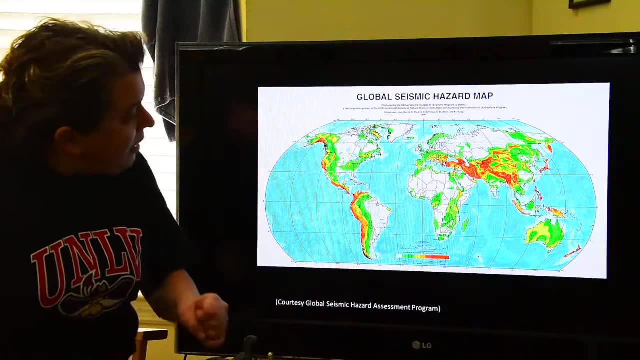 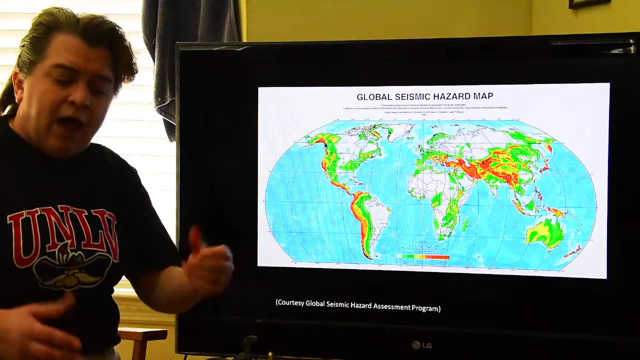 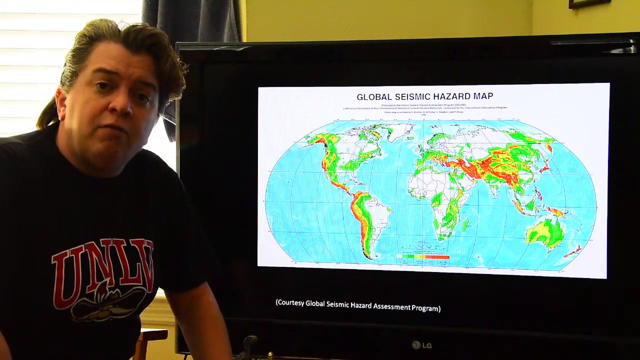 never happen in a place that's shaded in white. it's just that the probability, the likelihood of a strong earthquake happening there is much less. and if we look at where our strongest earthquakes tend to occur and where they happen most often, that corresponds with plate boundaries. the movement of the plates is one of the major things that causes earthquakes. but let's zoom in. 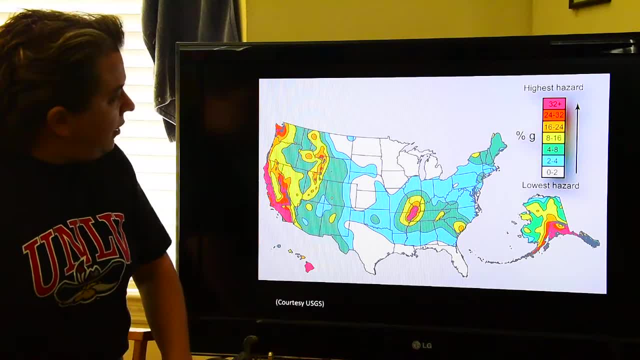 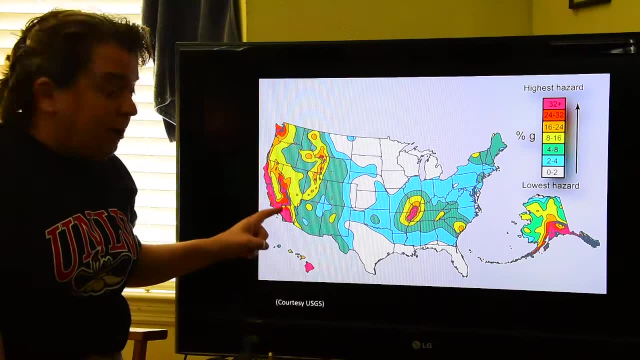 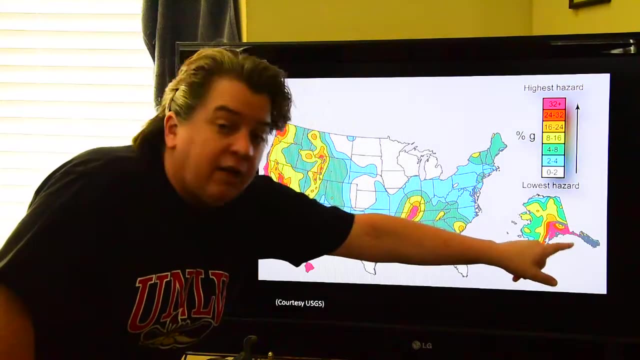 on the united states and we can see again: the highest hazards in the, the reds, the lowest hazards in the blues. the west coast of the united states, that's an active plate boundary, so that's where we get the most earthquakes up in Alaska, that's also a plate boundary. Hawaii is a little bit. 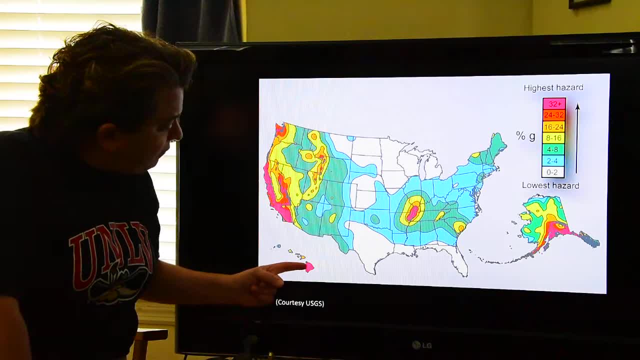 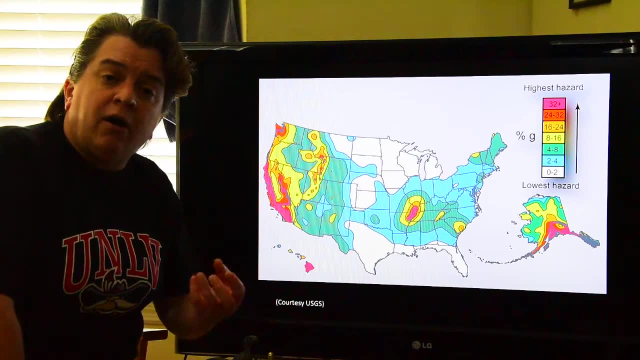 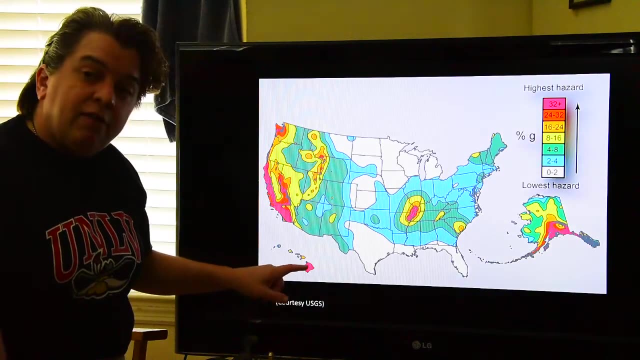 different, because it sits in the middle of the pacific plate, yet we see a high earthquake hazard, and that's because it is an active volcano and the movement of magma under the ground can also cause earthquakes, and so, even though that's not a plate boundary, that you can still have a higher. 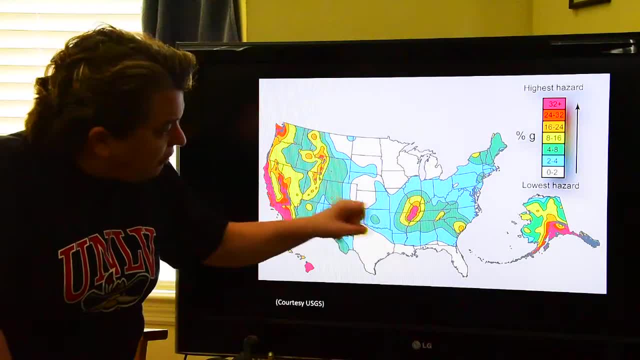 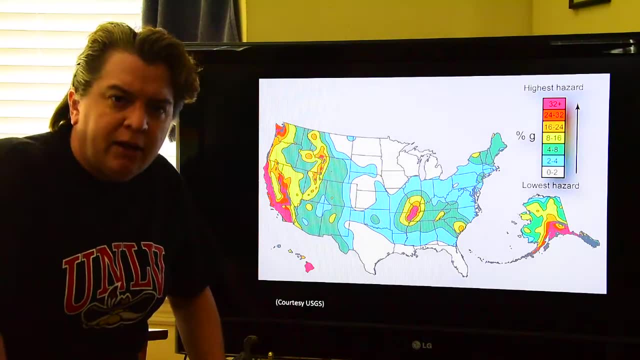 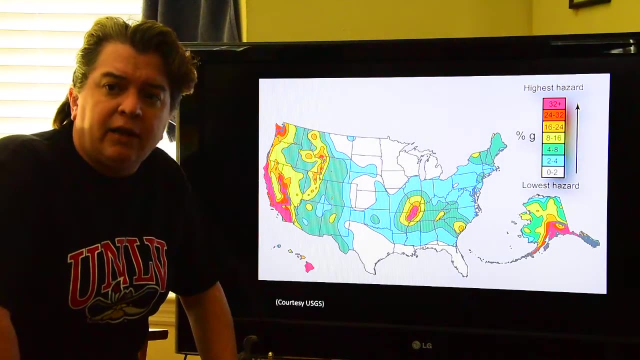 earthquake hazard there. but then we get these locations here which are in the middle of the North American plate, nowhere near any kind of plate boundary, and yet we have elevated earthquake hazards there. we call those intra-plate earthquakes, meaning in the middle of the plate, and why those happen is 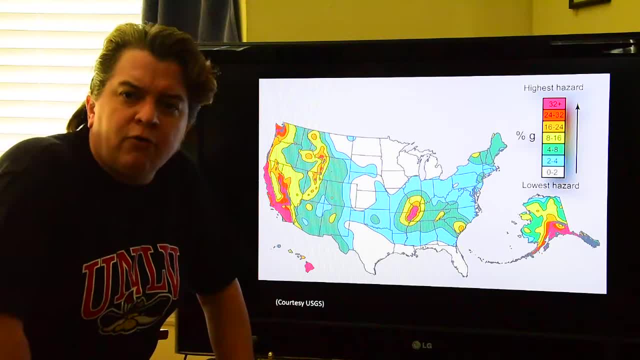 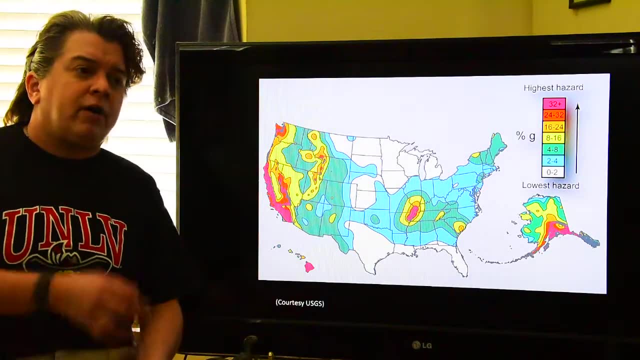 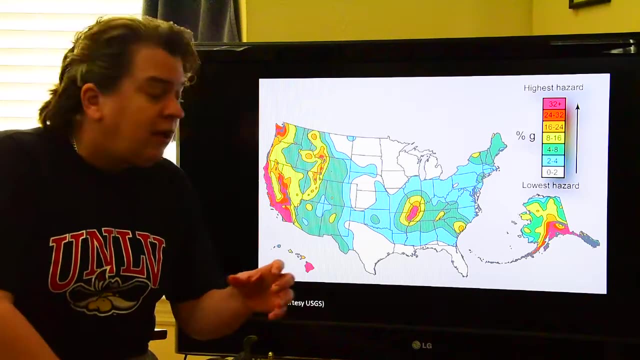 because while those are not a plate boundary today, at one point in time in the distant past those were plate boundaries, or at least they were places of active tectonics. there are still zones of weakness in the earth's crust that sometimes- not that frequently- but 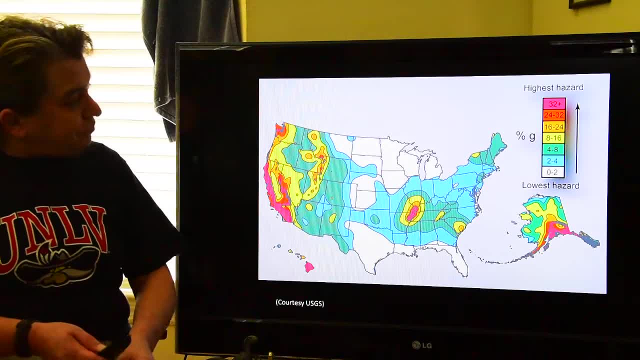 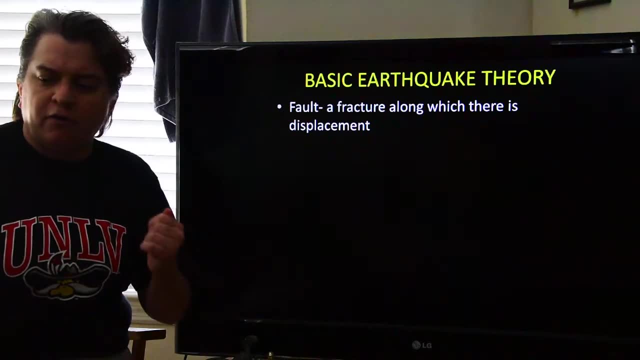 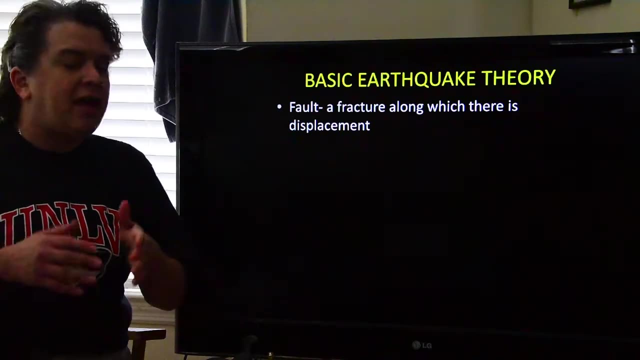 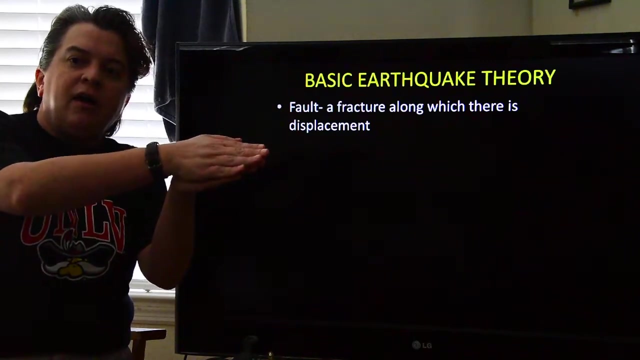 sometimes have strong earthquakes. all right, so let's take a look at why earthquakes happen, a look at our basic earthquake theory. so earthquakes typically happen along a fault, and a fault is a fracture in rocks along which there is displacement or movement. okay, so basically you have two rocks and they're cracked in two and on one side they're moving compared to 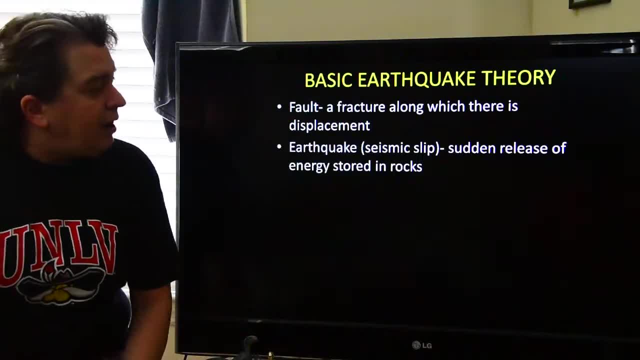 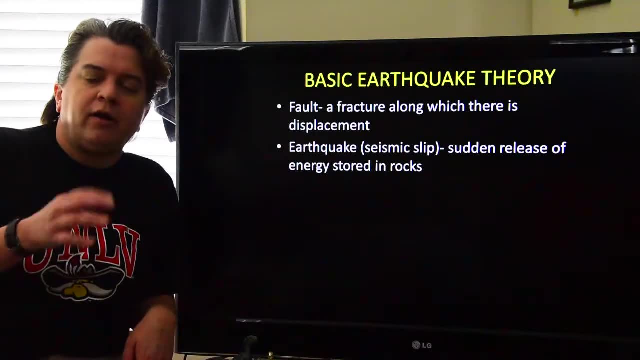 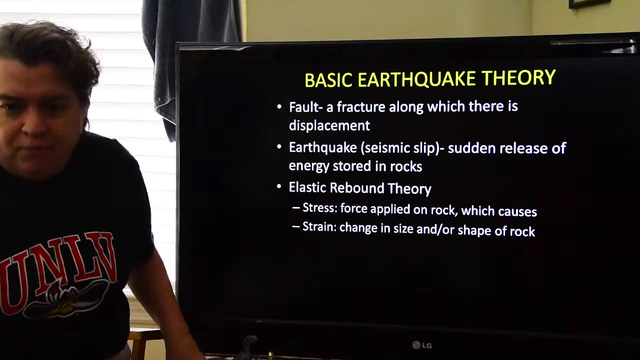 the other side. that's a fault. now, an earthquake, known as seismic slip, is the sudden release of energy stored in rocks. so, though, you might be sitting there asking: how do these rocks store energy? and it comes down to elastic rebound theory, and this is something that was developed. 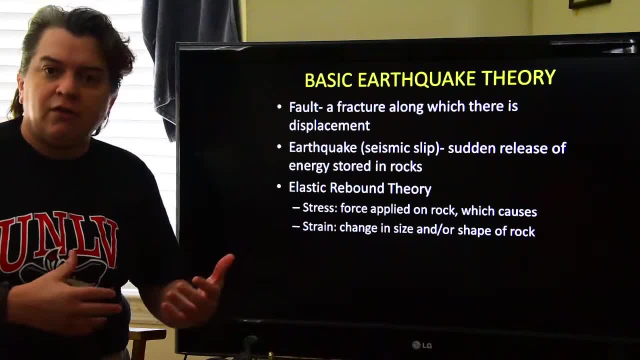 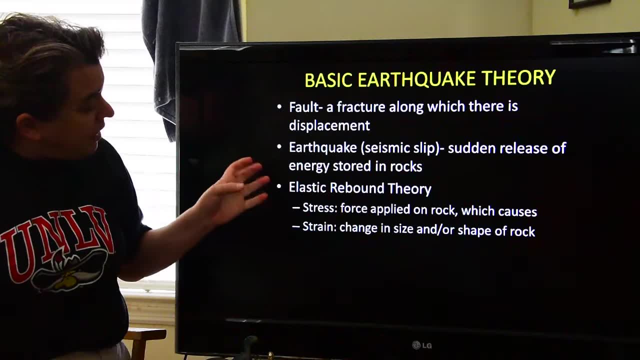 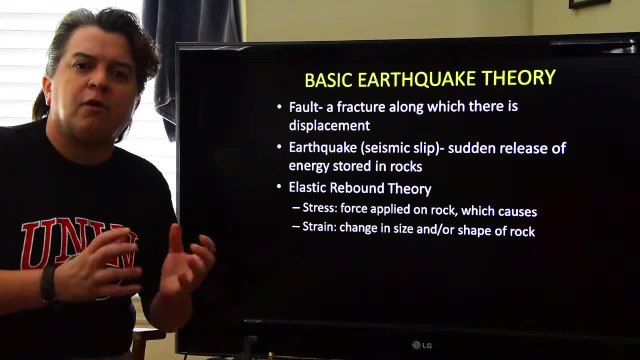 by geologists in the late 19th century- and this is the first earthquake that hit san francisco- geologists really worked on figuring out why earthquakes happen and they developed this theory at that time. and so elastic rebound theory states that we have a stress on rocks and stress is a 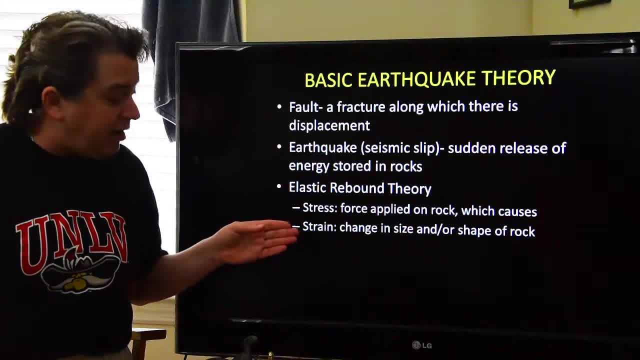 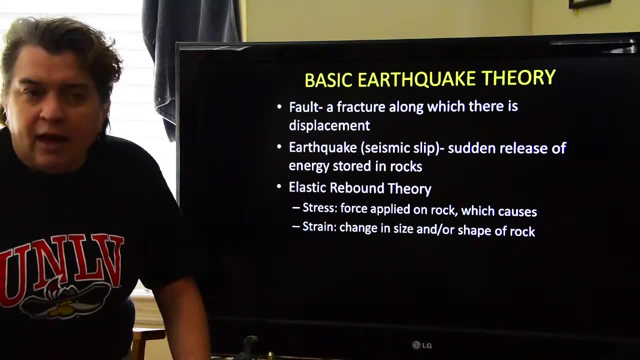 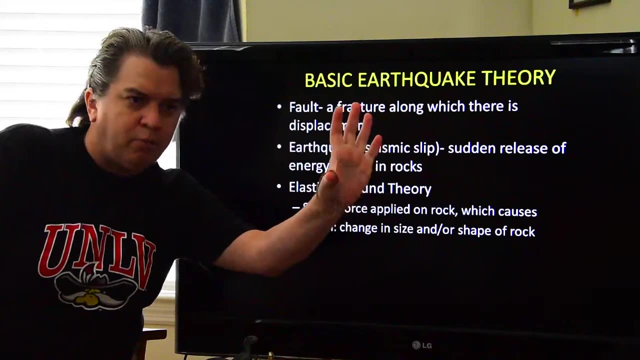 force applied to rocks, and that force applied to the rocks causes strain, and strain is a change in energy. and by the time we got to our 30th century and people thought, oh wow, it looks like we are not really talking about the heat, and all right, we're talking about a quartz. 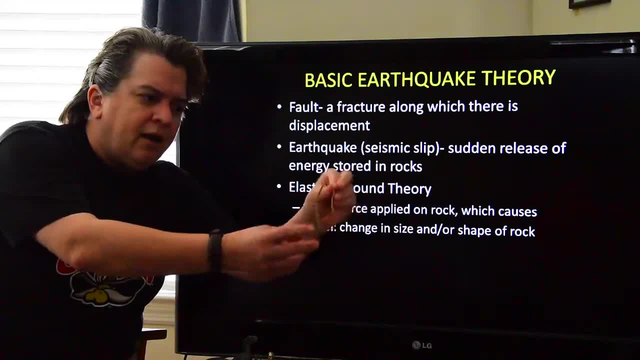 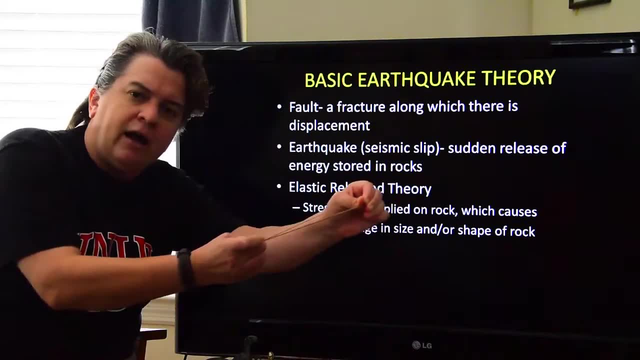 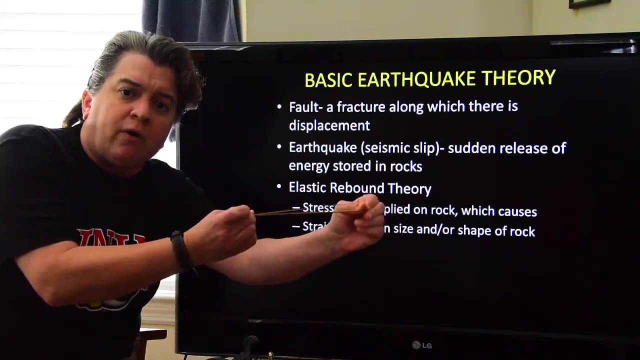 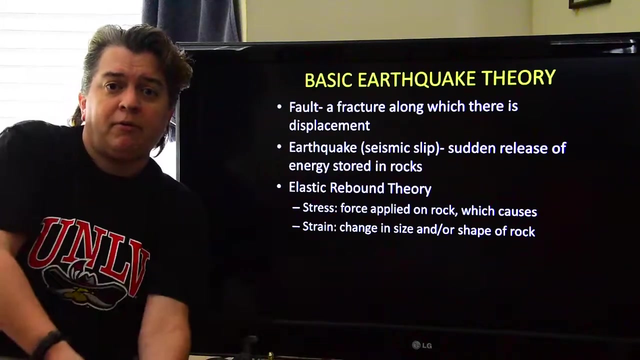 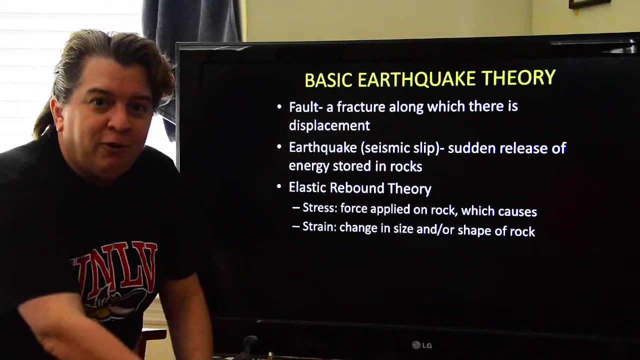 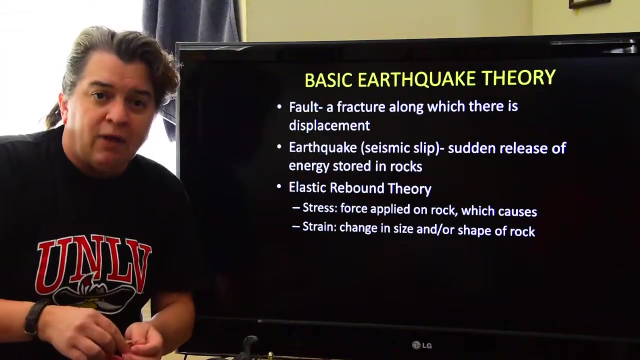 and then the earth is still going this way. so that's what we do right now about the earth be released heads up right. so when I let go of that, it flew right because the energy was being released and that's what allowed it to move like that and 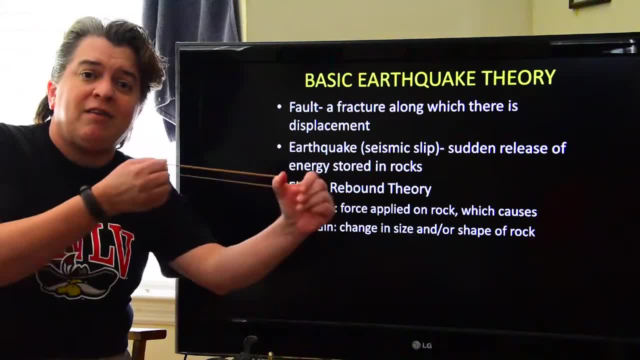 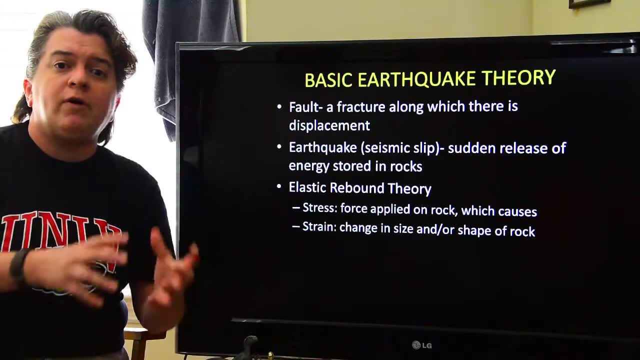 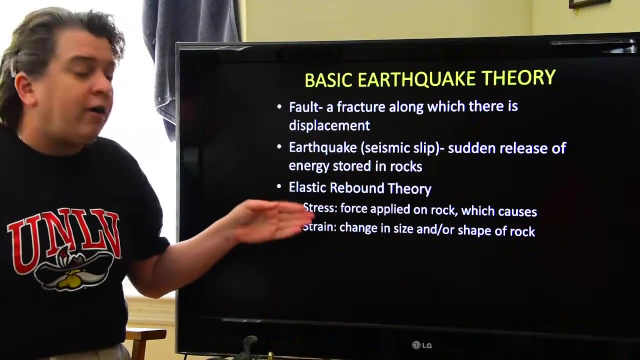 the same thing happens with rocks. now, rocks are not going to be as elastic as this rubber band, but when you do have these tectonic plates moving around, when you have forces applied to them, they are going to slowly get deformed. they are going to start storing energy that will ultimately be released as an earthquake. 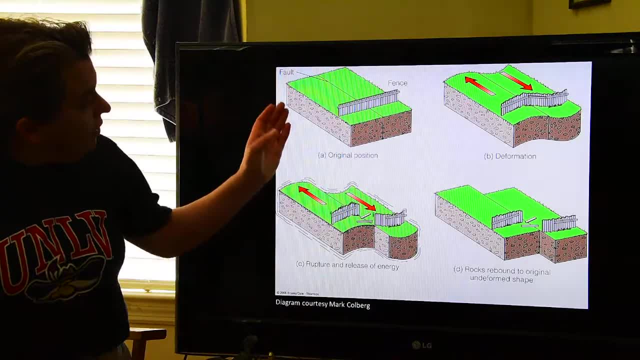 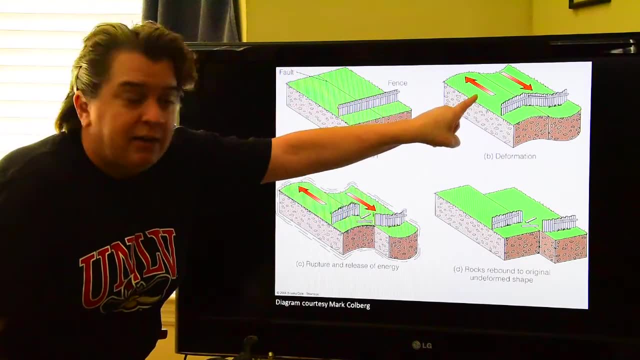 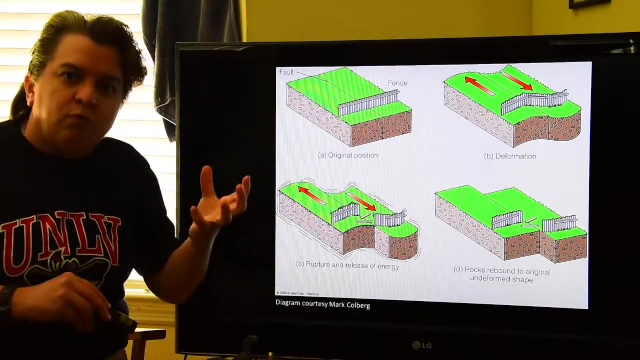 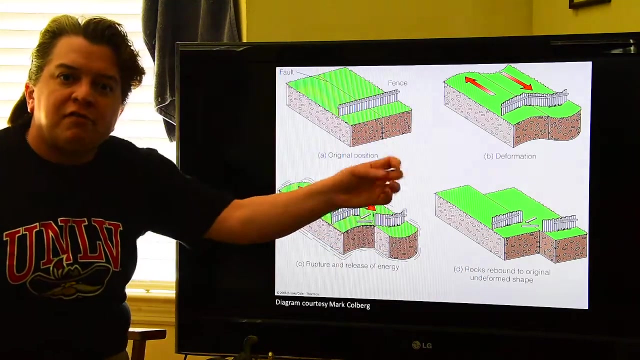 and that's what this diagram is trying to show. here's our original rocks. there's the fault. now we have our forces applied to that, and so the rocks are getting bent and deformed and eventually they're going to rupture, which is basically the release of that energy, and they get back to their original size and 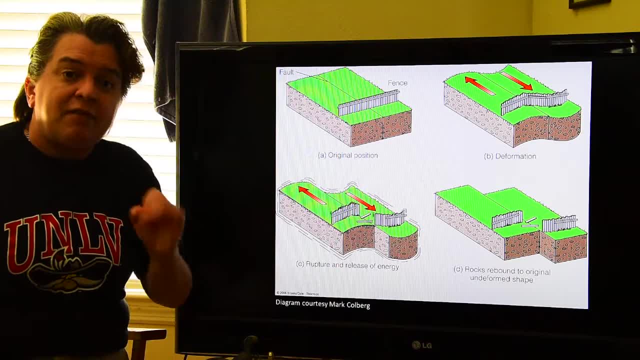 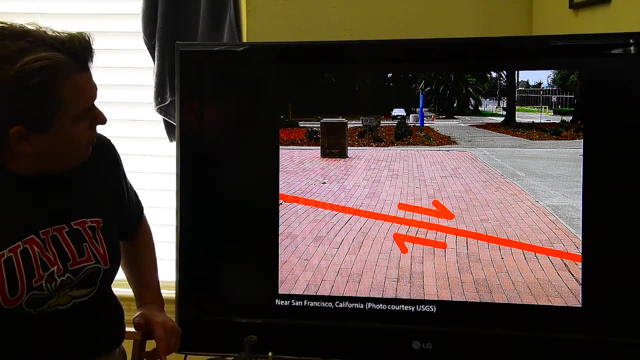 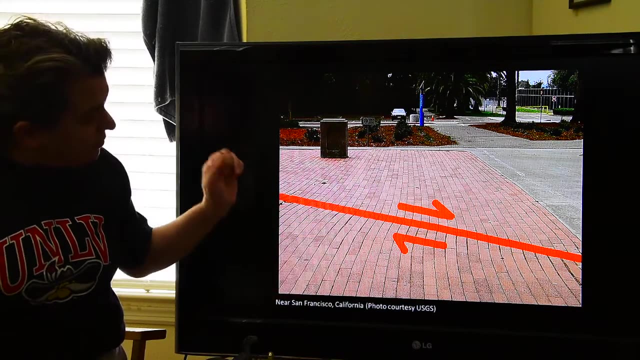 shape after releasing that energy, and that's elastic rebound. now what we are seeing right here, this is in San Francisco or somewhere around San Francisco and notice how these bricks are a little bit bent. that's because this is built right across a fault where we have this slow movement of the fault. 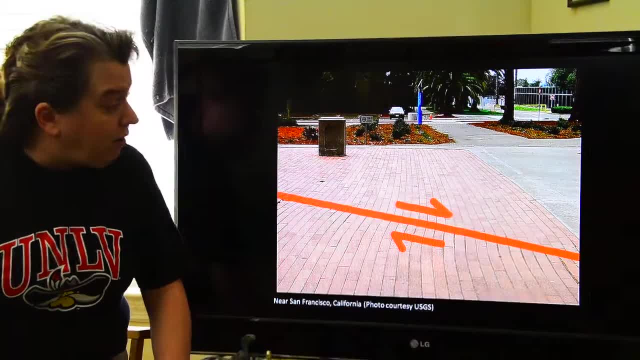 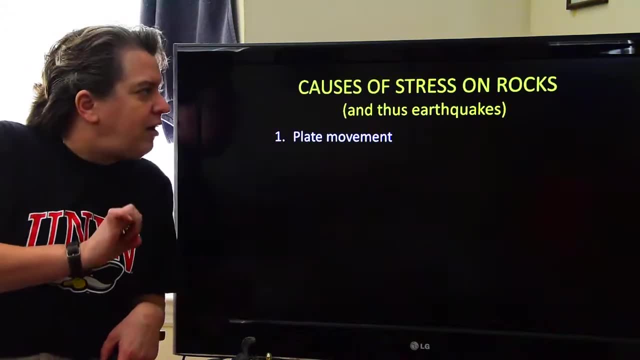 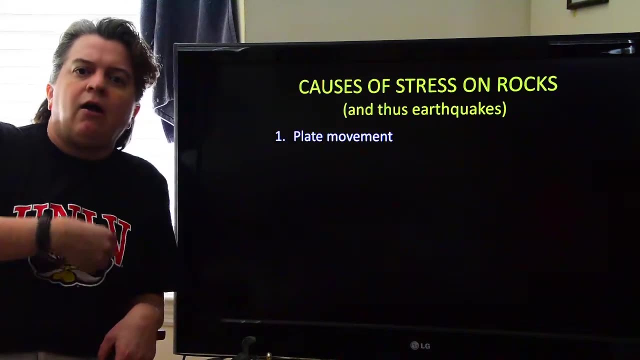 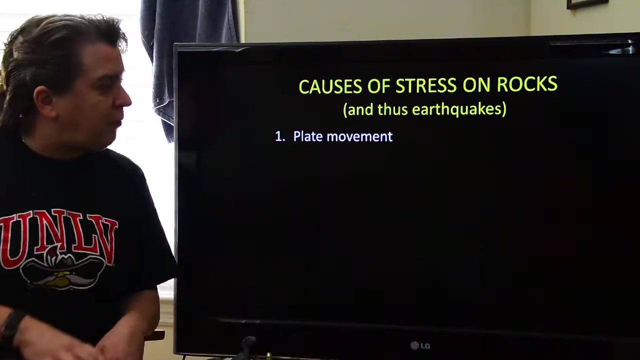 that is deforming the, the rocks and thus the bricks right there. so, then, that leads us to ask the question: well, what causes stress on rocks? if stress is what deforms the rock, that ultimately leads to the earthquake, what causes stress on rocks and thus causes earthquakes? well, the big one is plate movement, right as 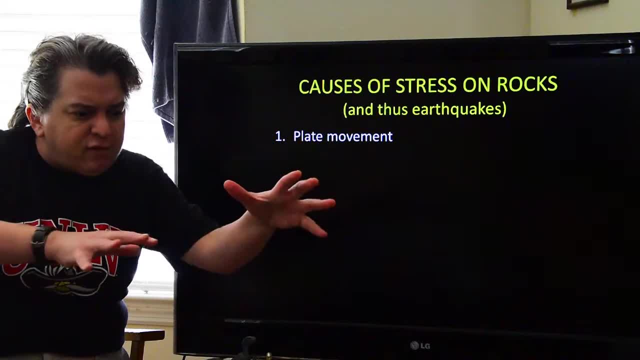 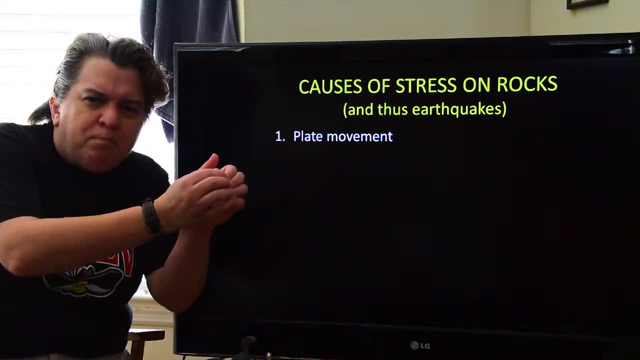 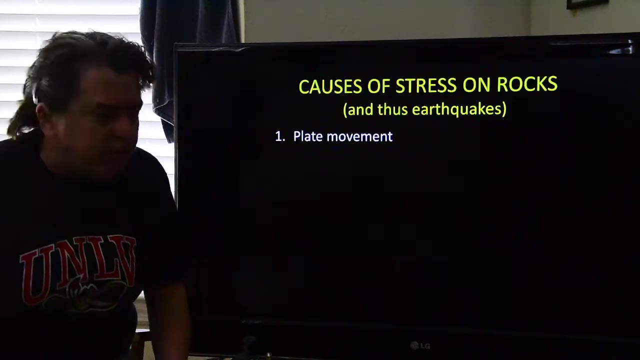 those giant tectonic plates are slowly moving and shifting around on Earth's surface. you know they'll catch against each other and and and bend and and deform each other a little bit, building up that enter, that stored energy in those rocks. but we can also have explosives, especially like big, massive explosions. 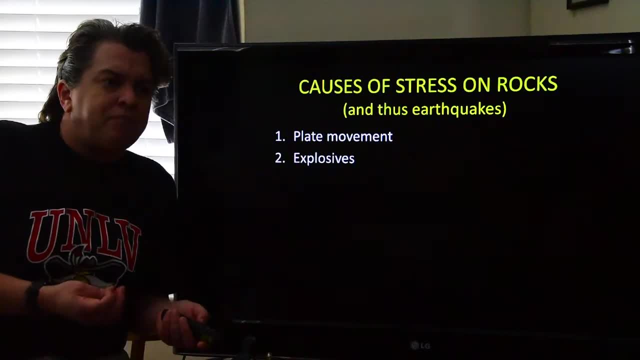 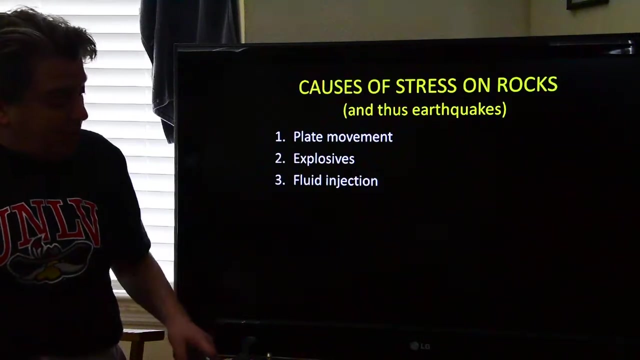 are going to cause earthquake waves. one of the ways people knew that or know that nuclear testing is going on is because when you test a nuclear weapon, it creates seismic waves that can be recorded all over the world. fluid injection can cause earthquakes, so fluid injection often times a way to get rid. 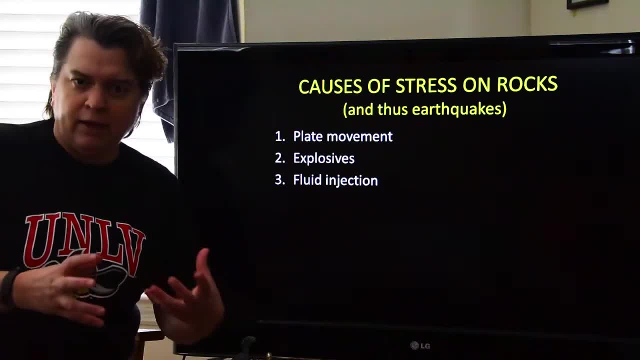 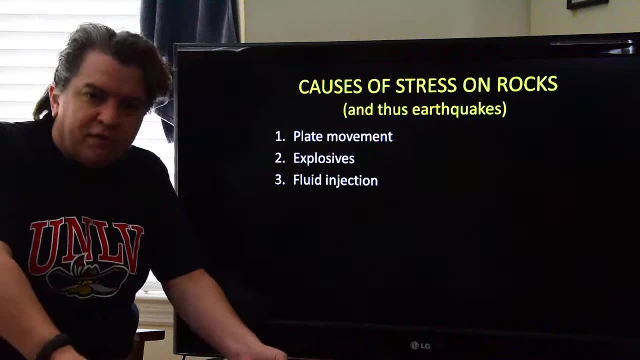 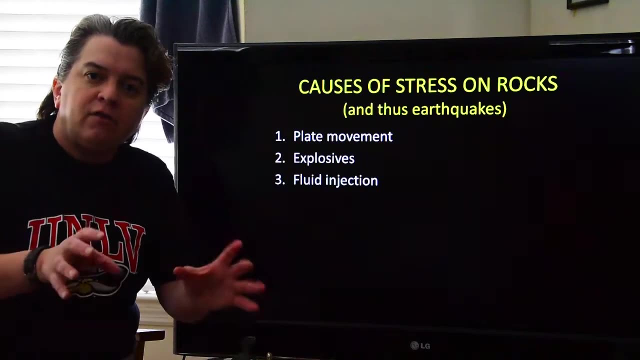 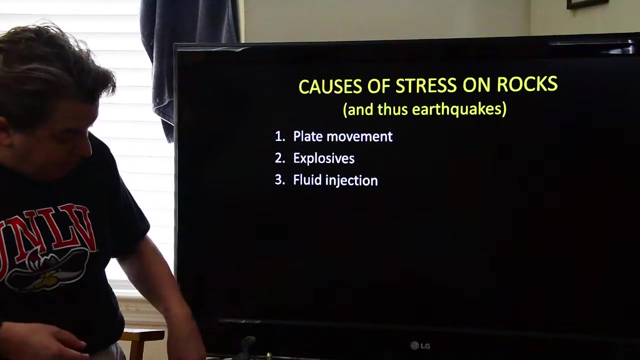 of hazardous waste, or really nasty waste, is to drill a deep, deep well into a rock, a deep hole, and then force the nasty fluids, the hazardous or toxic fluids, deep underground into those rocks. like I said, we are forcing them into the rocks right. so that's going to create our strain, our deformation on the rocks and 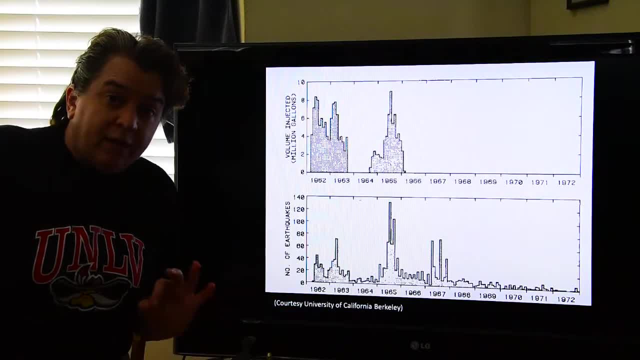 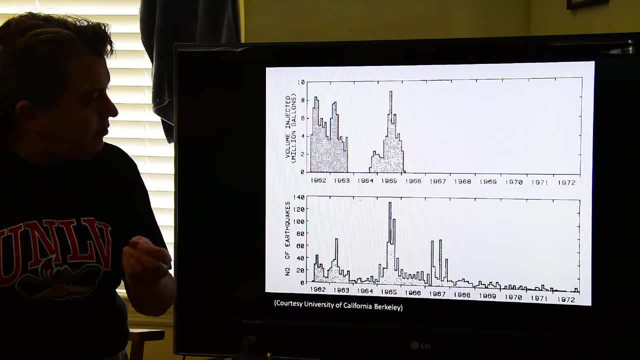 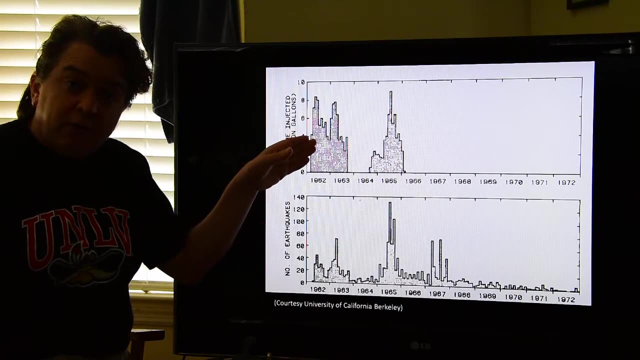 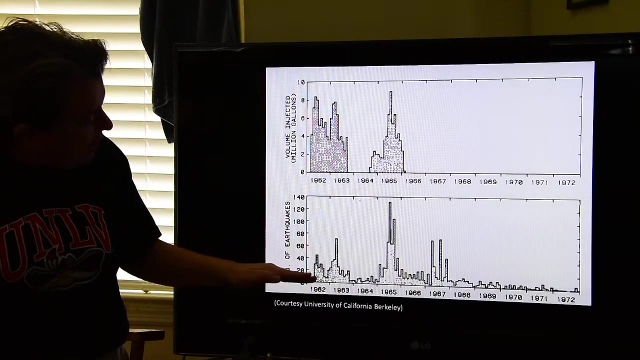 ultimately can lead to earthquakes, and one of the classic examples that's being used of that goes back to the Rocky Mountain Arsenal back in the 1960s. what we're looking at here on the top is fluid that was injected underground. the higher the the bar, the more fluid that was injected. and then down here we're. 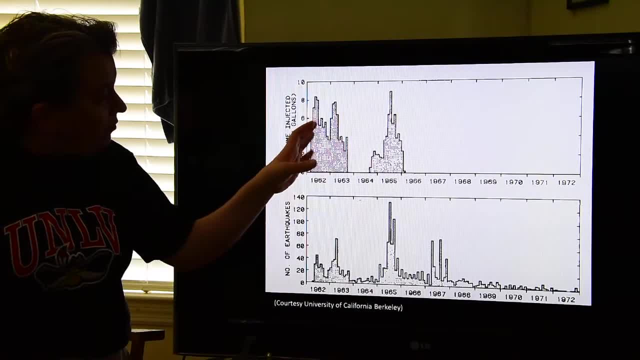 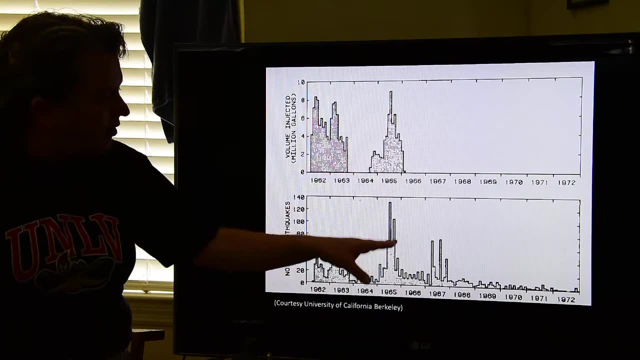 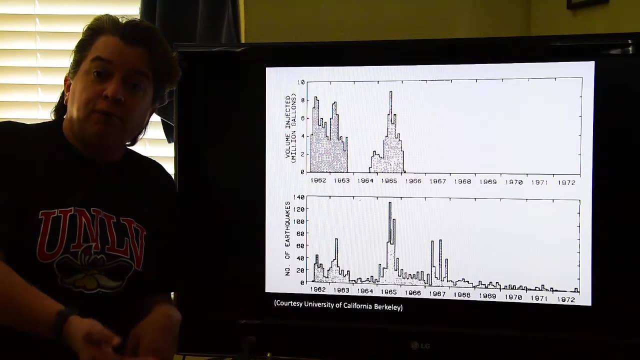 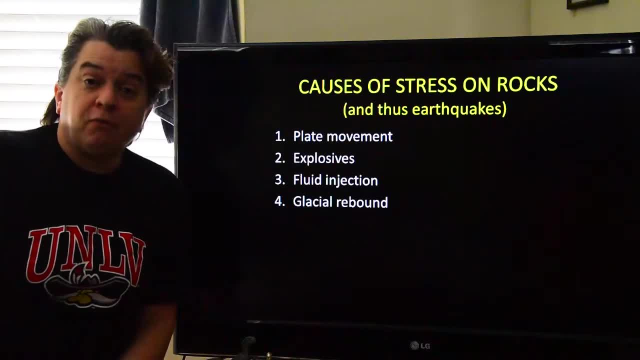 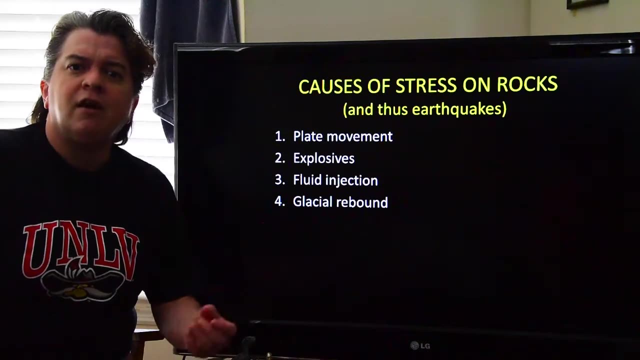 earthquakes and that is a reason why in some places where they have to get rid of fracking fluid, that you will have an increase in earthquakes in places in parts of Oklahoma and parts of Texas and actually some other states that didn't have a lot of earthquakes before had more. 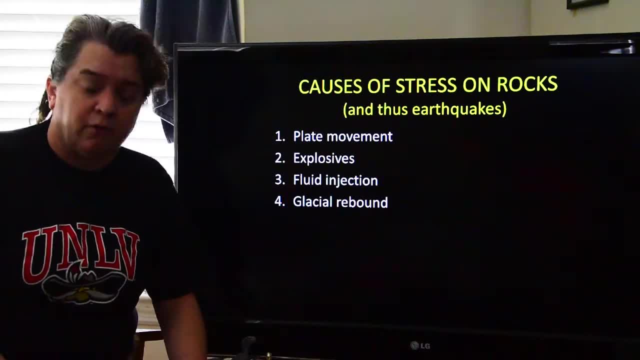 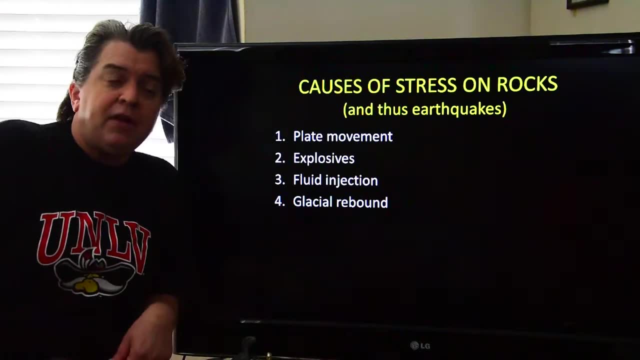 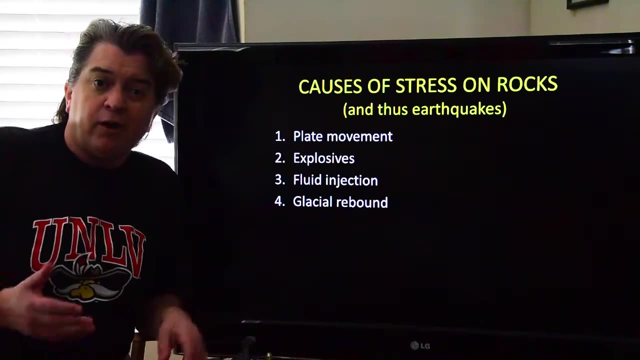 when they started disposing of those fluids deep underground. all right, another reason why you can have earthquakes is glacial rebound. so glaciers are these, these big, thick masses of ice, and they weigh a lot, right, one gallon of water weighs bit over 8 pounds. now imagine you have a piece of. 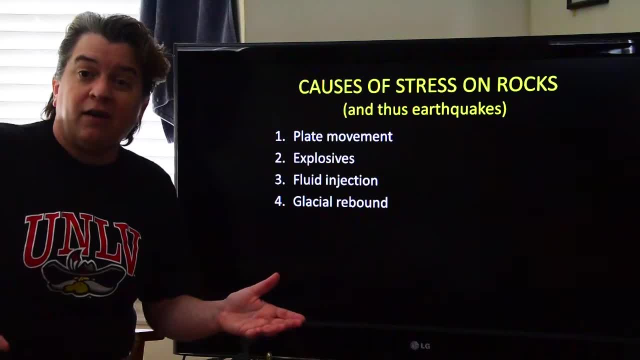 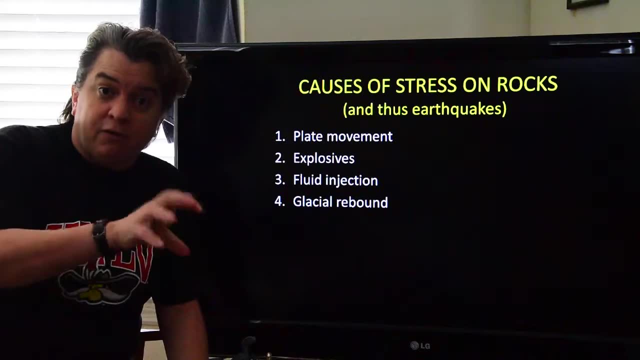 ice, that's three or four tons of ice, and you have a piece of ice that's three or four kilometers thick. right, that's gonna be a lot of weight on Earth's crust. and remember that gooey asthenosphere underneath Earth's lithosphere. well, if 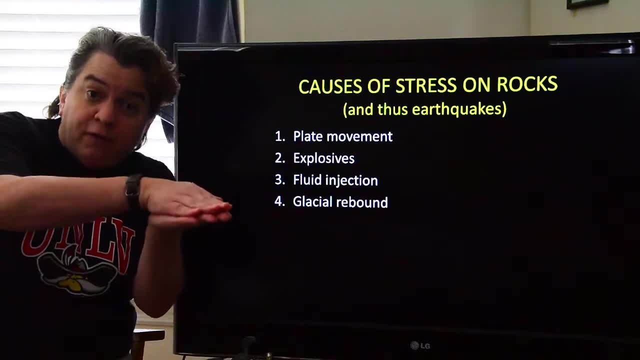 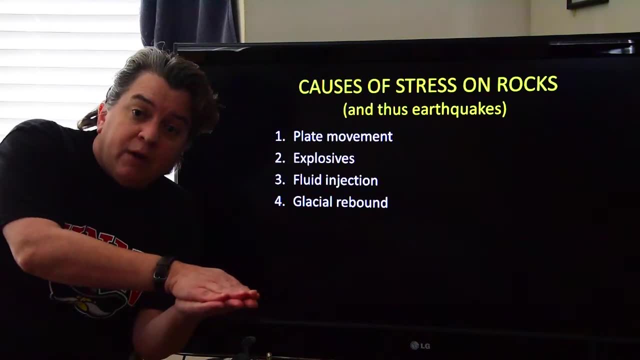 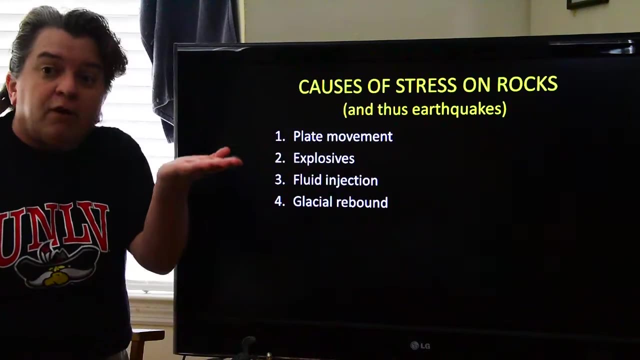 we have a whole lot of weight on the lithosphere. like that glacier, it actually pushes the lithosphere down into the gooey asthenosphere. but if that ice melts there's nothing pushing it down anymore, so the lithosphere will start rising back up and down and it's really very difficult to see the ice. 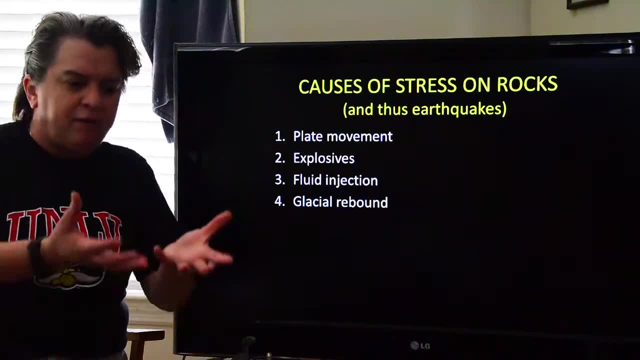 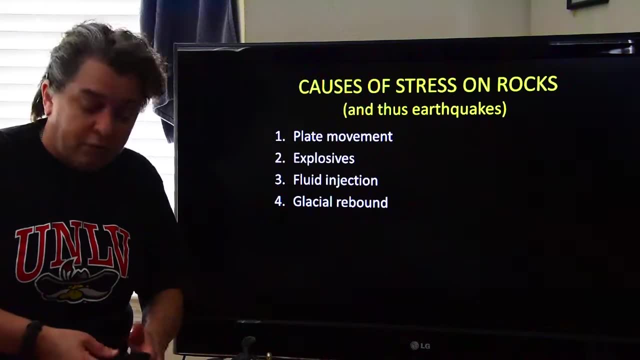 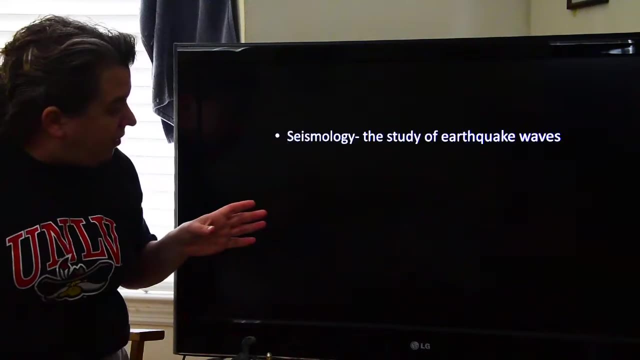 back up. that's called glacial rebound, where that lithosphere rises after the glaciers go away, and this movement can actually trigger earthquakes in some places. now these are things that can- volcanic activity, by the way, also can trigger earthquakes, and there are some other things, but really the most common. 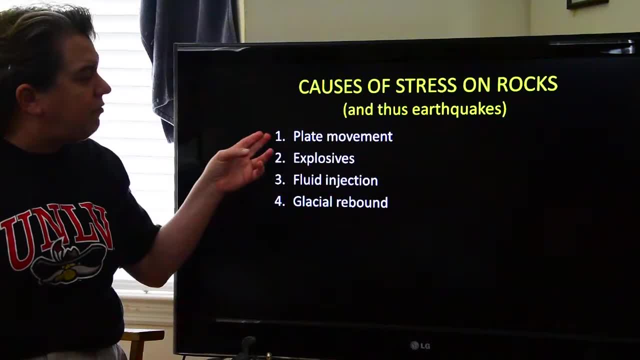 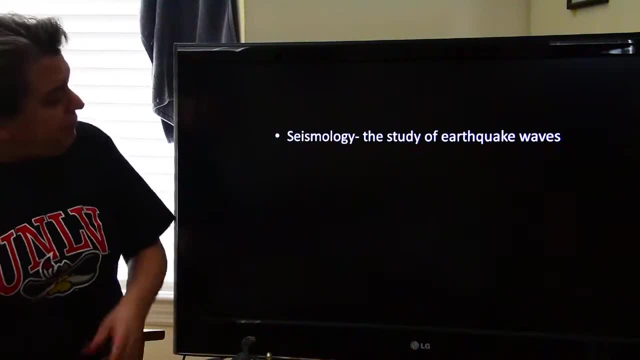 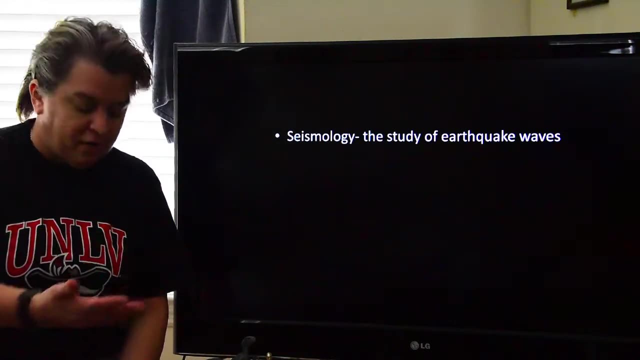 cause the most. the common thing that's going to cause earthquakes is the movement of the plates around Earth's surface. all right, so seismology. seismology is the study of earthquake waves. right, I already said seismos means shaking, ology is study, so it's actually kind of the study of shaking. well, it's. 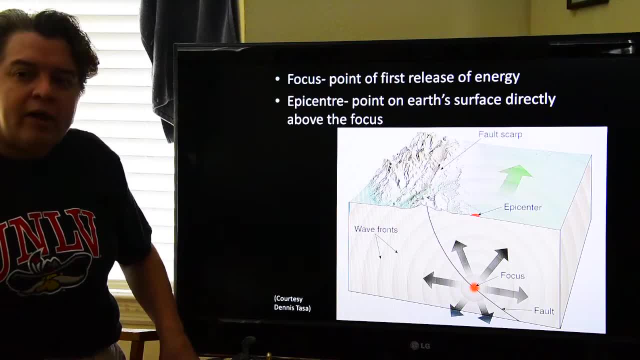 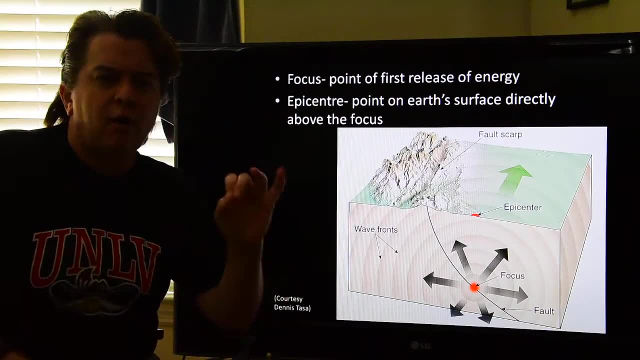 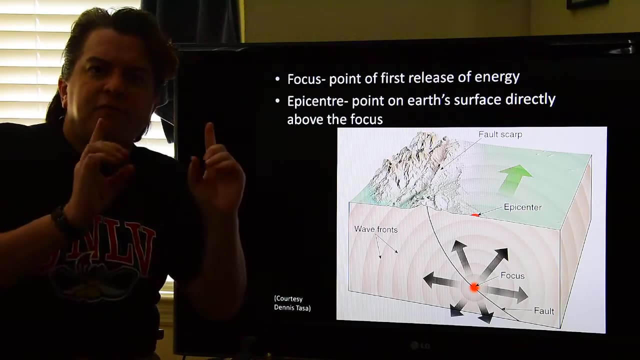 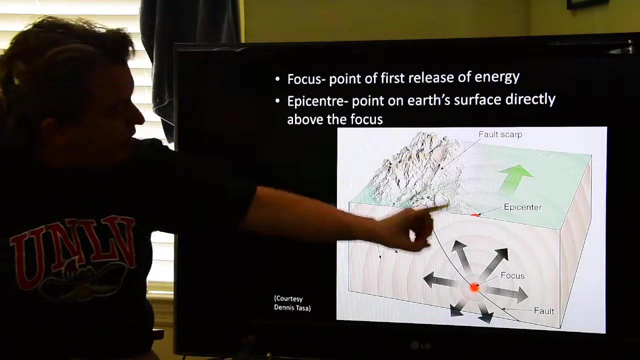 the study of earthquake waves and when we are looking at earthquakes and an earthquake happens, I said that's this release of energy that was stored in the rocks. well, the place where the energy is first released in an earthquake- so you can think of it as like the place an earthquake starts- is the focus and 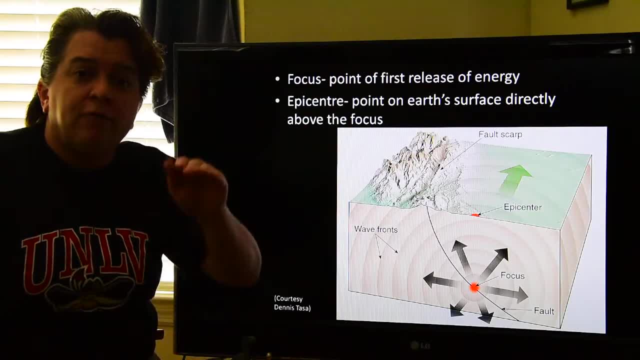 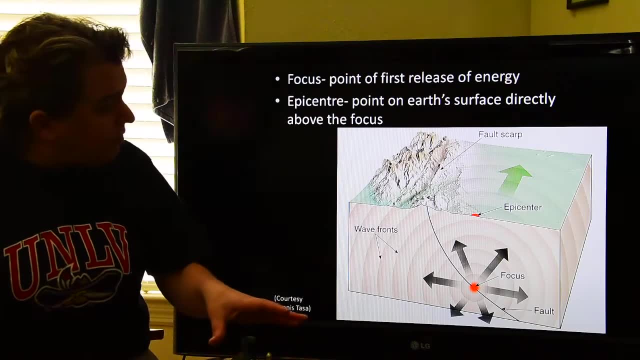 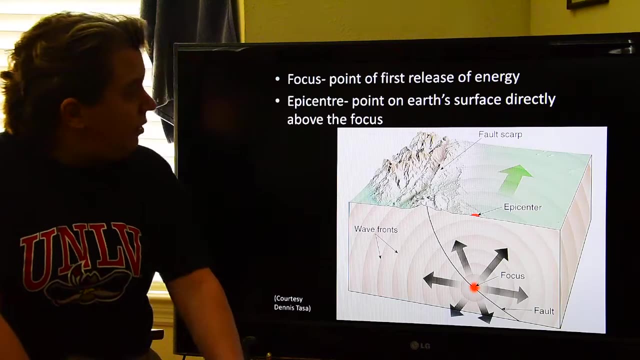 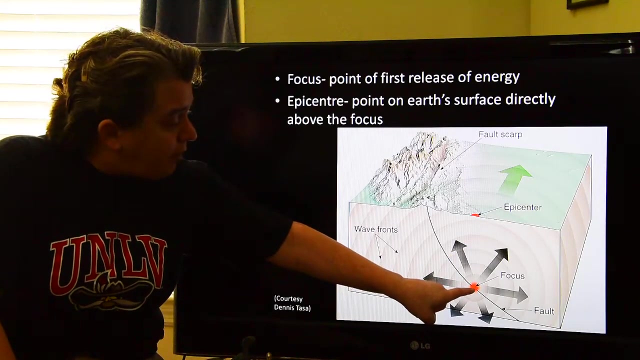 the focus can be anywhere from Earth's surface to around 660 kilometers deep. you don't usually get earthquakes much deeper than that. now you've probably heard the term epicenter. well, the epicenter is the point on Earth's surface directly above the focus. so what we're looking at in this diagram here faults. 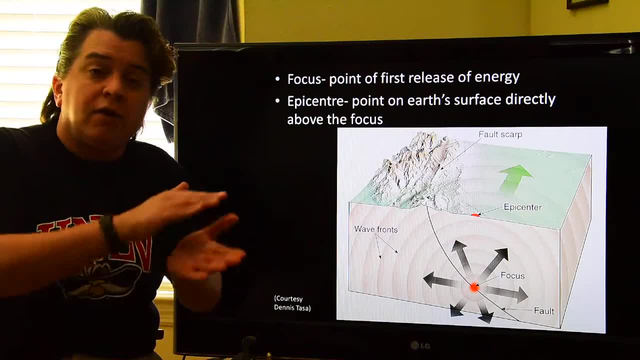 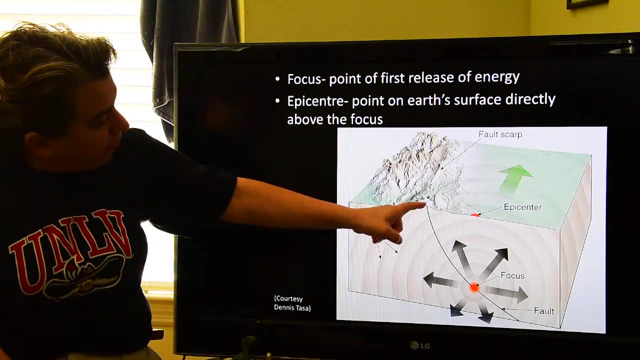 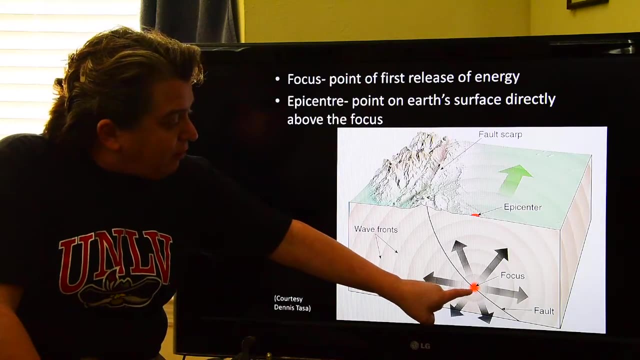 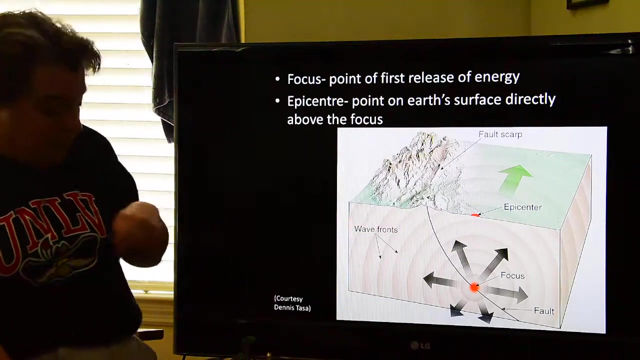 are three-dimensional surfaces right. they're not just a line on a map, they go underground. so here's the fault on Earth's surface, but there it is underground. so in this case, the first release of energy in the earthquake was right there. so that's the focus, and then right above it on Earth's surface, that's going to be the 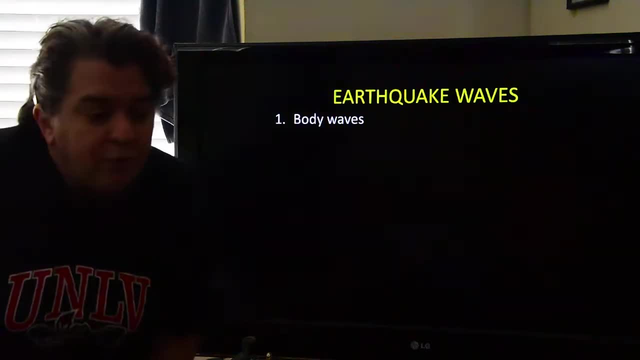 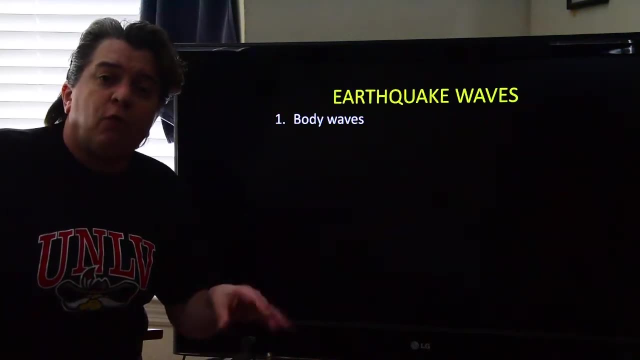 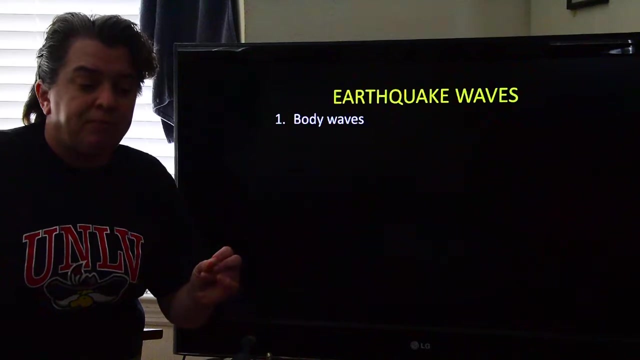 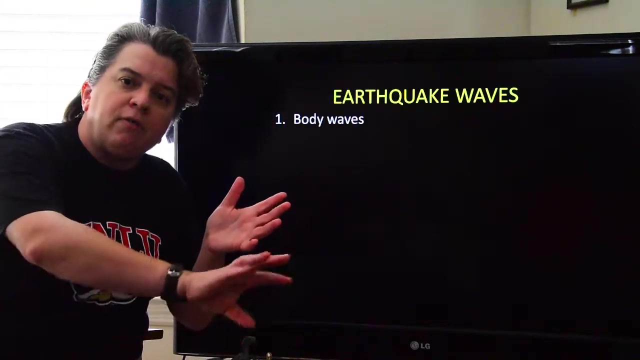 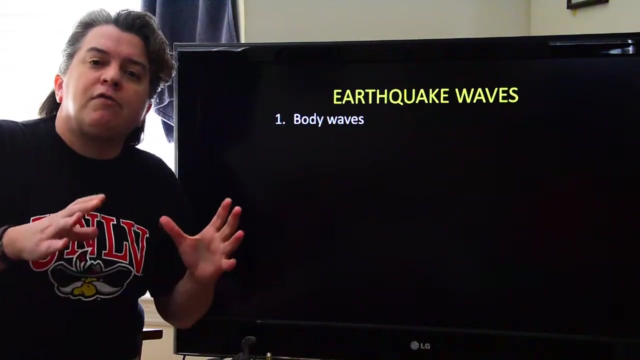 epicenter. now, when waves, when, when the earthquake occurs, the way this energy is released is in the form of waves, and four different earthquake waves are released. two of them are body waves. body waves will travel all the way through the center of the Earth and right they go through the Earth's body. and then there's also what are called surface waves. 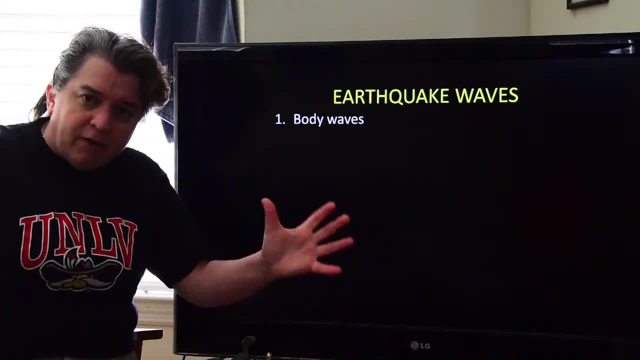 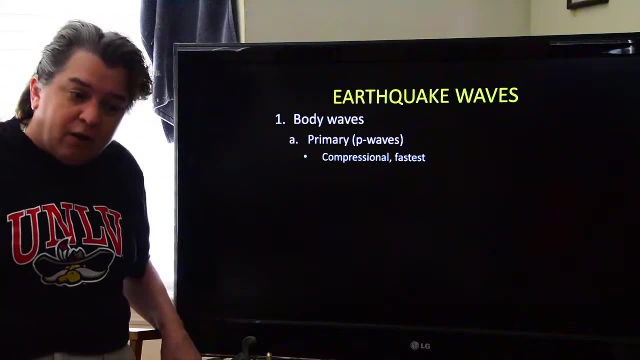 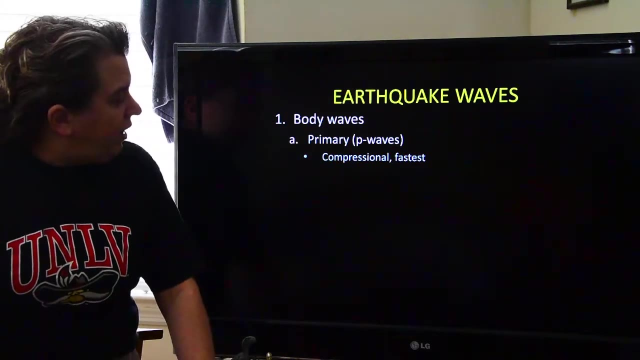 and surface waves basically stick around Earth's surface and can travel all the way around the surface. so let's look at these body waves first, these ones that go through the planet. there are what are called primary waves, and Primary waves are abbreviated P waves, and P waves are compressional. 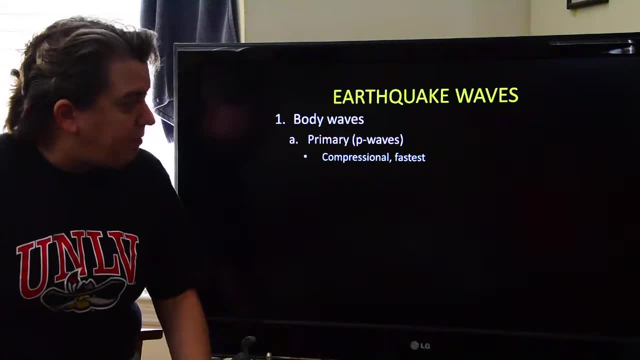 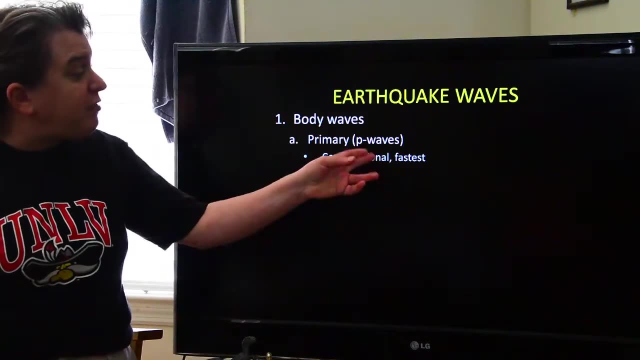 They have kind of this push-pull movement to them as they travel through the Earth. These are the fastest earthquake waves. In fact that's why they're called the primary waves, So if the earthquake happens in one place and you are in another place, 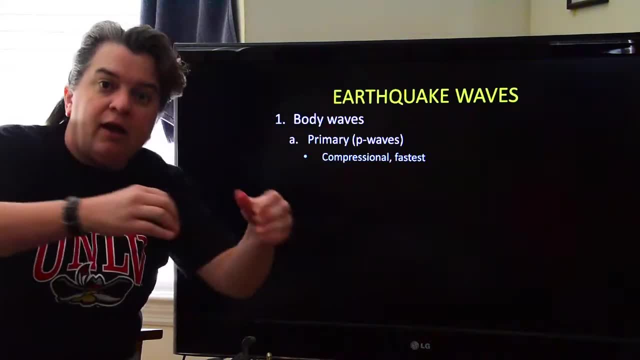 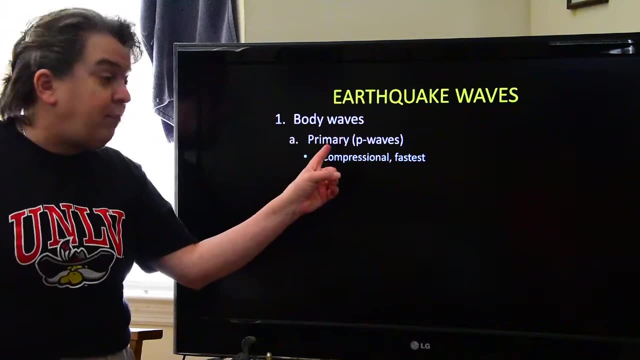 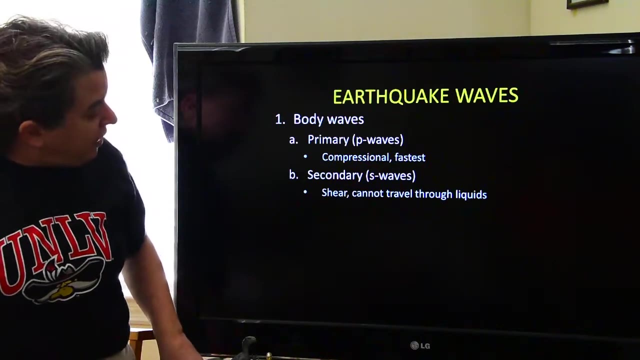 those earthquake waves travel to where you're located. The ones that travel the fastest are going to be the ones you feel first. Primary means first, So they're the first ones that you're going to feel Now. the other body waves that you have are secondary waves. 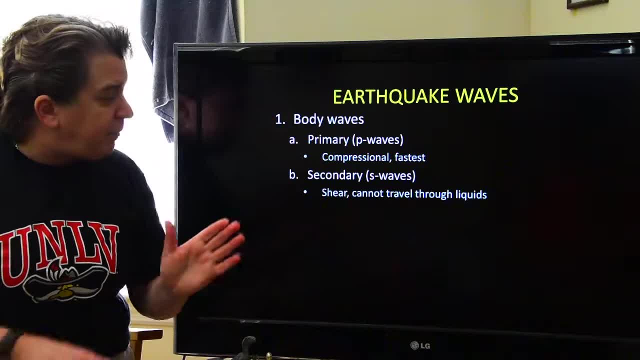 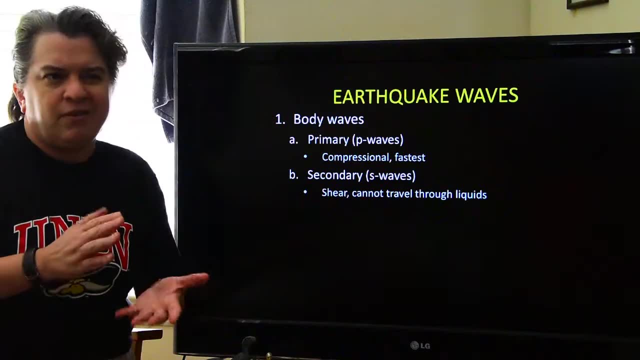 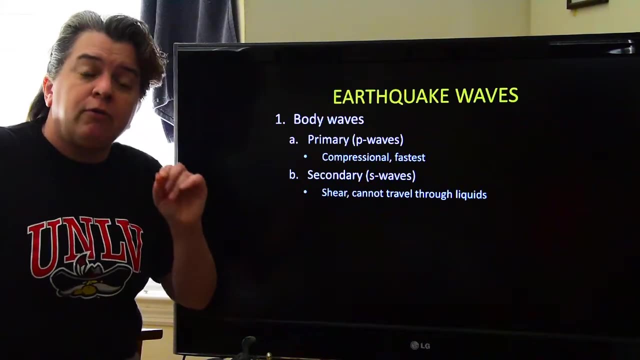 Secondary waves move through Earth a little differently. Instead of that push-pull motion like the primary waves, these have a shear motion. You can think of it kind of as almost an up-and-down motion, And these secondary waves cannot travel through liquids. 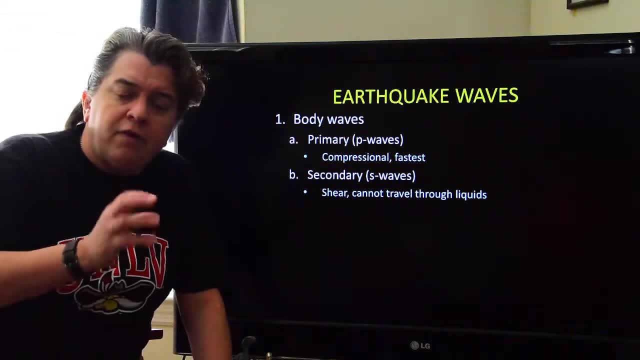 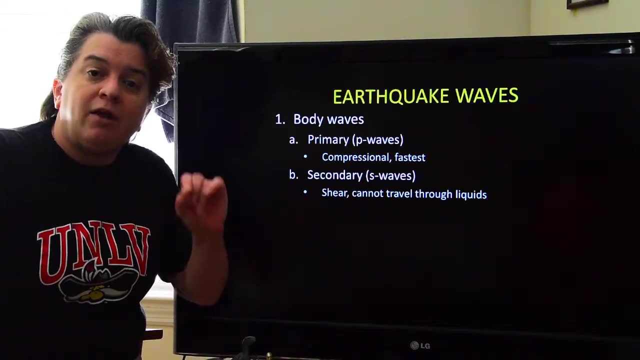 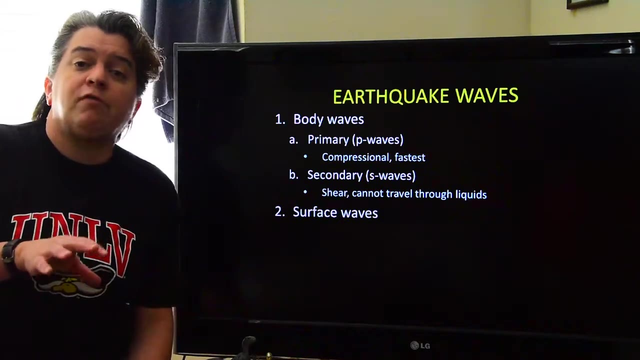 So earlier, when we were going over Earth's interior, I said the outer core is liquid And the reason we know it's liquid is those secondary waves can't travel through the outer core. Now, in addition to those body waves, we do have the surface ones. 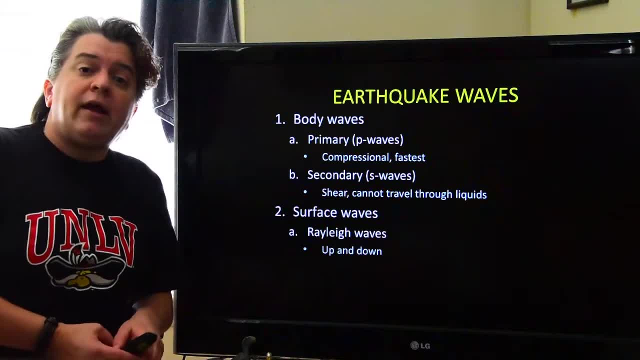 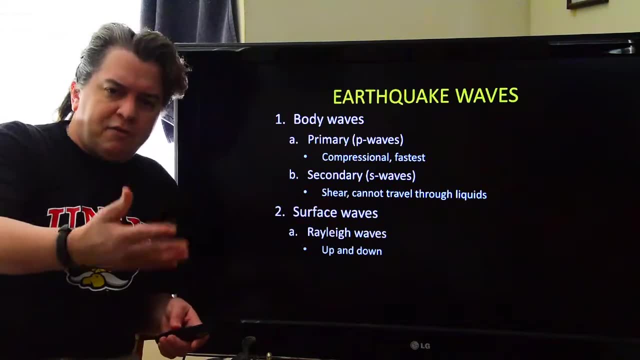 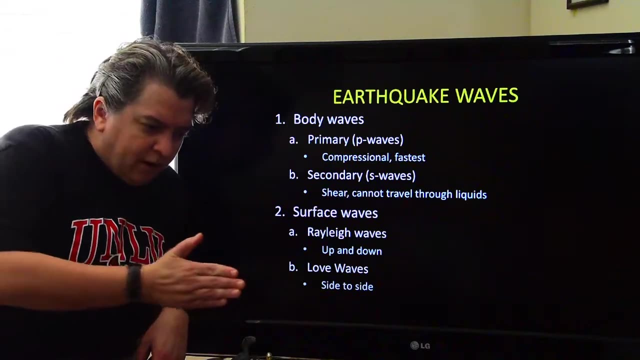 And in the surface waves we have what are called Rayleigh waves. Rayleigh waves have kind of an up-and-down motion, almost like ocean waves as they move. And then we have the Love waves, And Love waves as they move forward, they move side-to-side. 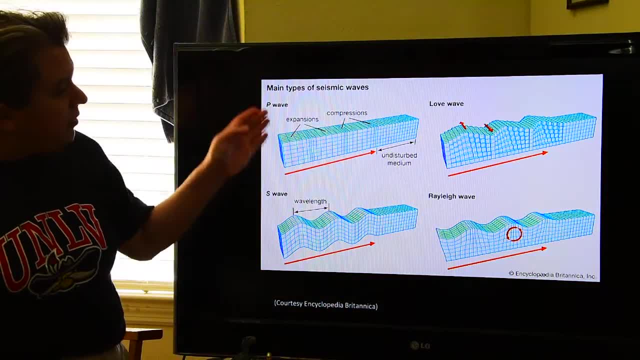 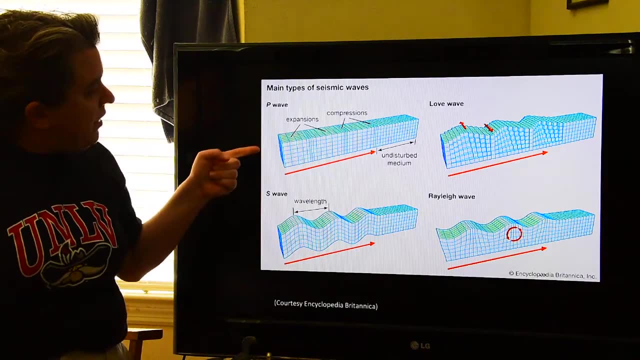 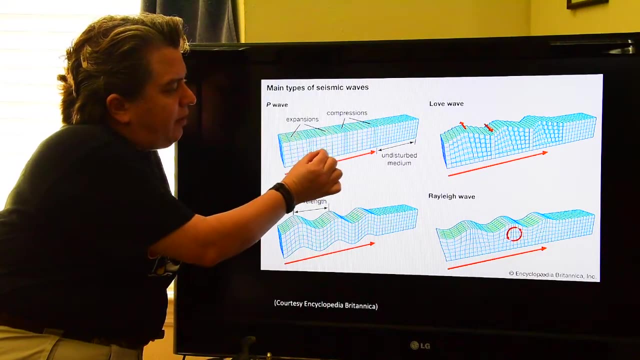 And I can show you this right here. Here's our main types of waves, Here's the body waves, Here's the surface waves, And so here's our P wave. Remember I said it's push-pull, So some places get kind of squeezed together and some places get a little pulled apart. 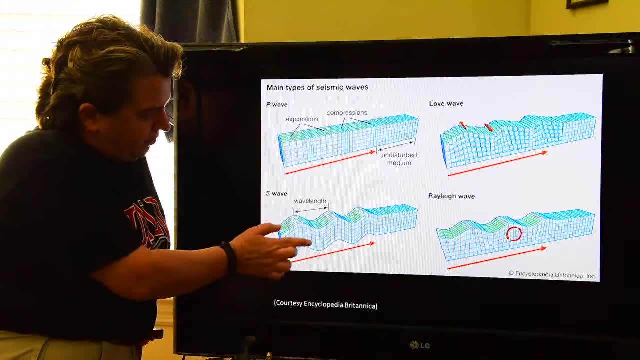 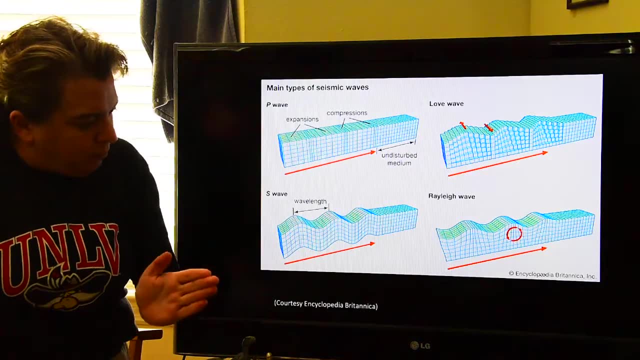 There's our S waves, right, So these are kind of side-to-side motion a bit more. There's our Love waves, Again, as they move forward kind of side-to-side, And there's our Rayleigh waves, which are much more like ocean waves. 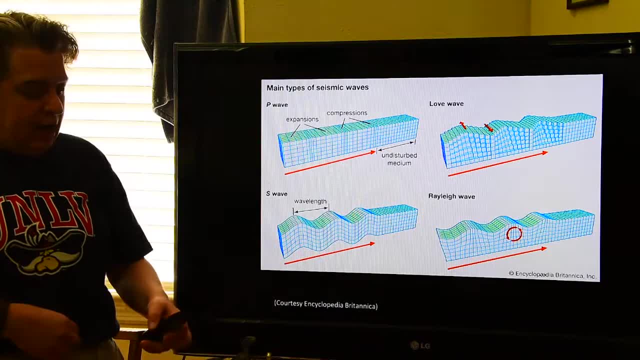 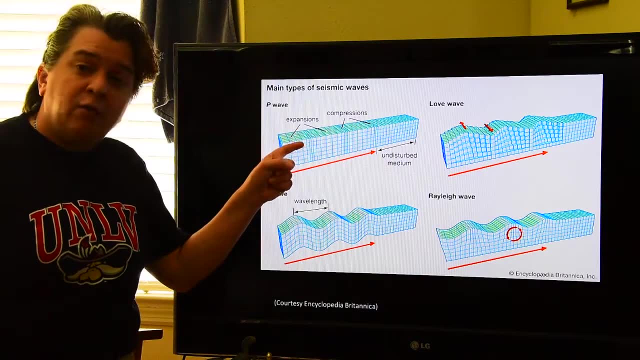 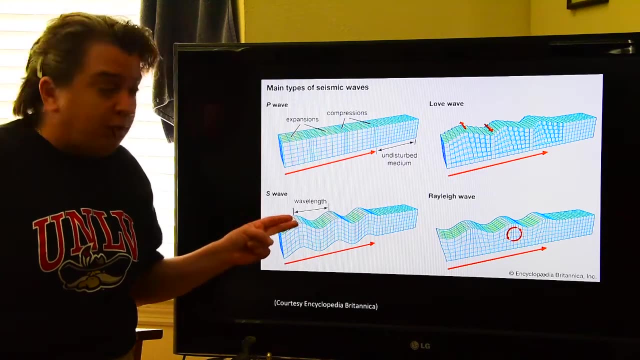 That kind of up-and-down movement that you would have. And when these are traveling through the Earth they do have different velocities. I said the P wave is the fastest, so that's the first one you'll feel. Then the secondary wave, the S wave, will arrive. 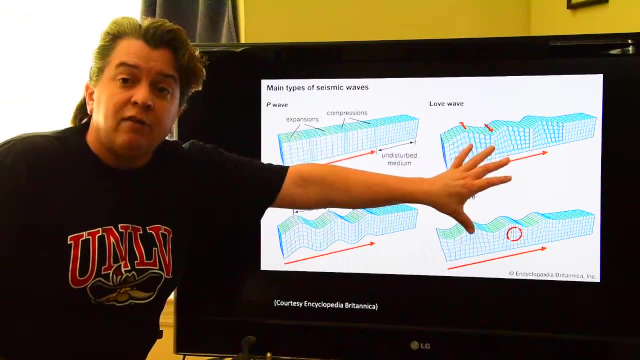 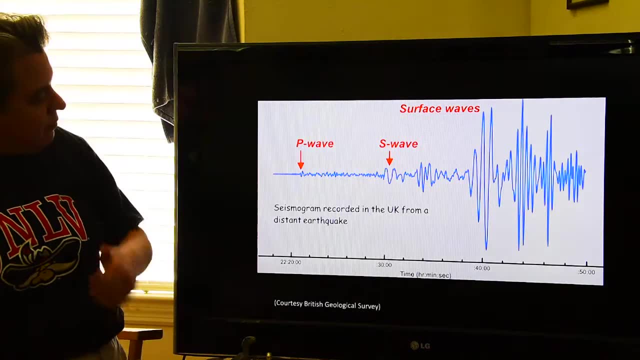 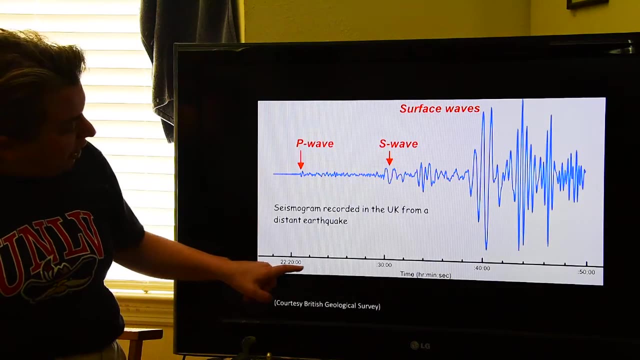 And then these are the slowest, And so those two will be the last ones that will arrive wherever you are feeling that earthquake, And that's what we can see right here. This is a seismogram from an actual earthquake, And you can see time down here. 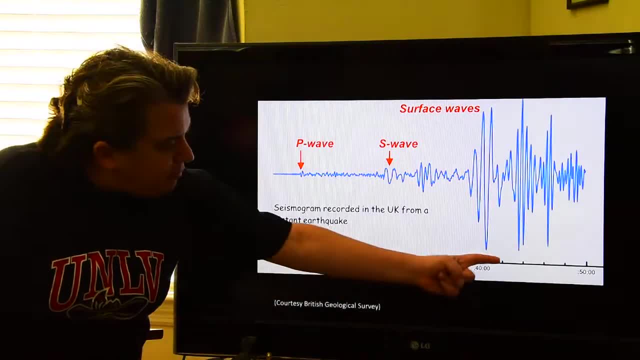 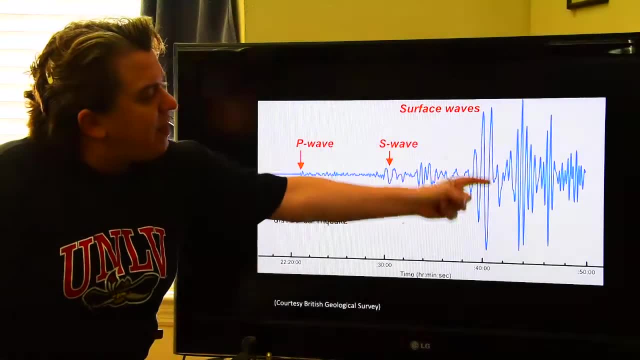 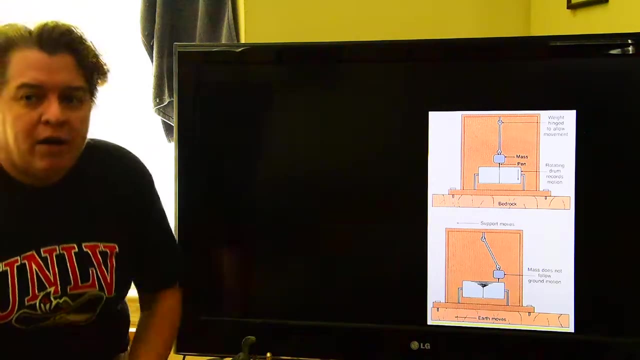 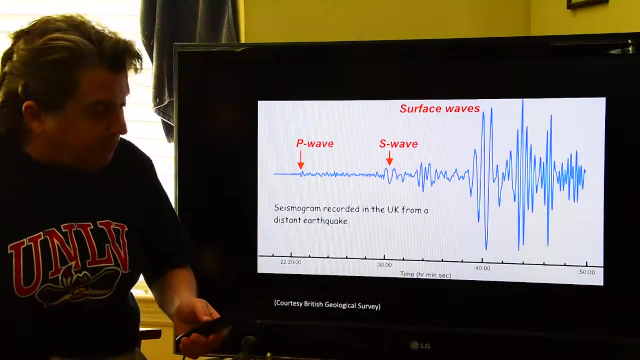 So this is the earliest time, And time is passing going in that way. So here we have: the P wave arrives, Then the S wave arrives, And then the surface waves arrive. Now, the way that we measure an earthquake and the way we get one of these weird little squiggly line things- 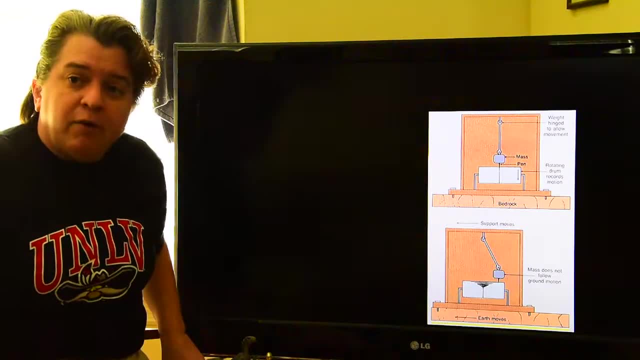 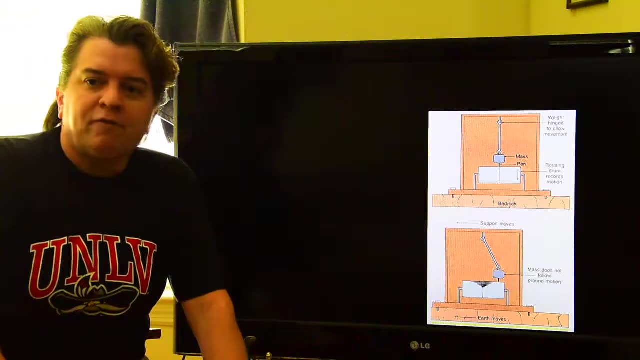 the seismogram. the way we get that is a seismograph. A seismograph creates that. It measures these earthquake waves, And this is an old-fashioned version of a seismograph, But it does get the point across of how it works. 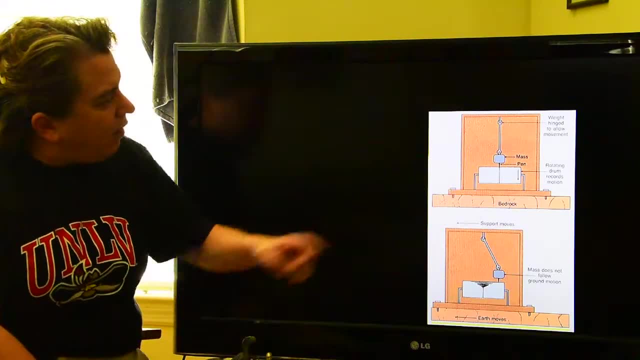 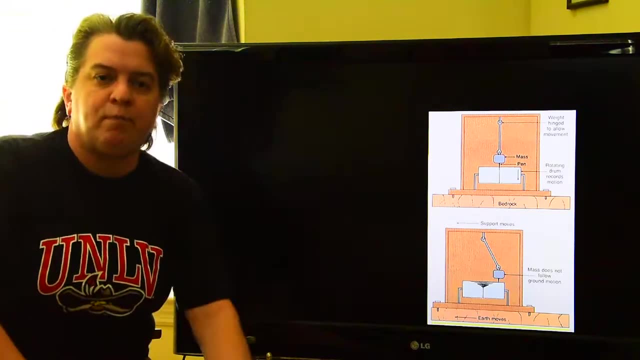 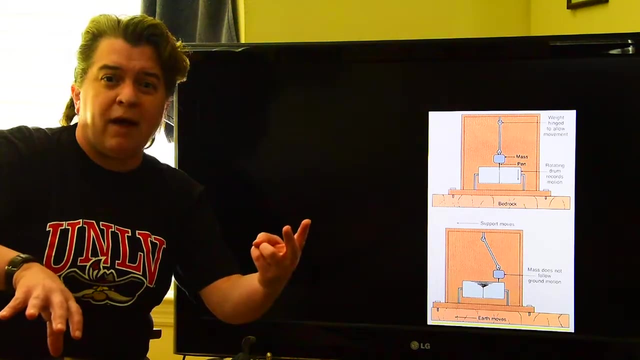 So basically, we have this box that's bolted into bedrock And inside that box we have this rotating drum, this rotating cylinder covered with paper. And I know everyone's seen this, because if you watch any kind of Hollywood movies where, like either aliens arrive or something bad is about to happen, 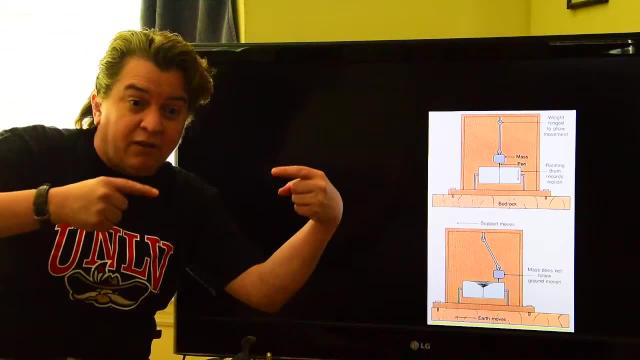 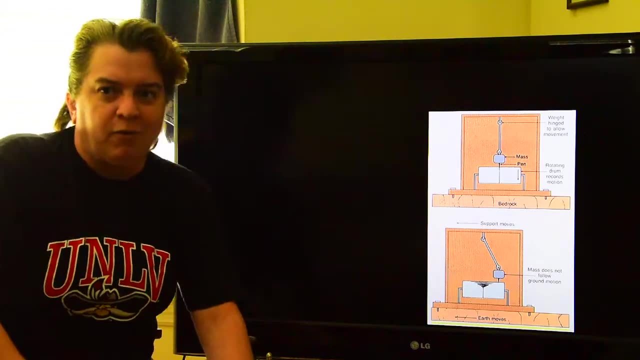 you see that piece of paper covering a cylinder that's slowly turning And there's a pen And right before the bad stuff happens, it starts really, really squiggling. That's a seismograph, And so that's in there. 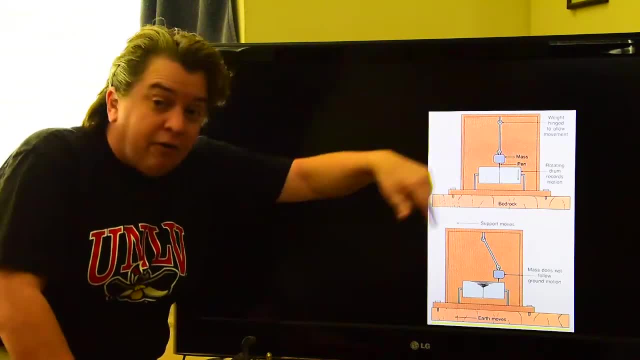 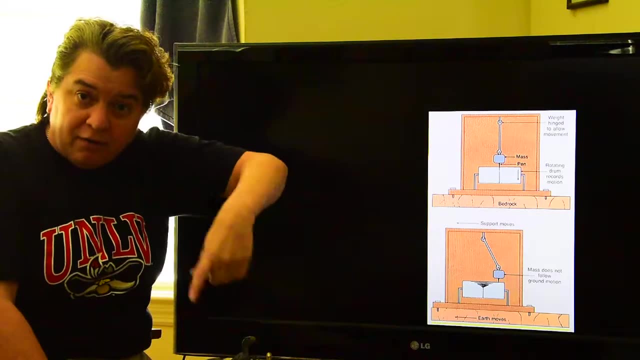 Now inside this box we have a pen right that's drawing the little squiggly lines. There's a big, heavy mass on that And this is hanging from the top of the box, So it's free-hanging. So how does this work? 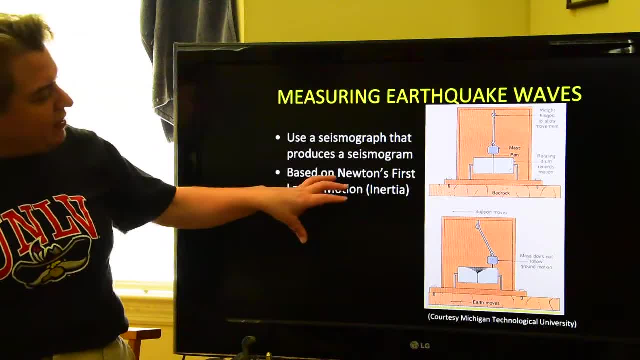 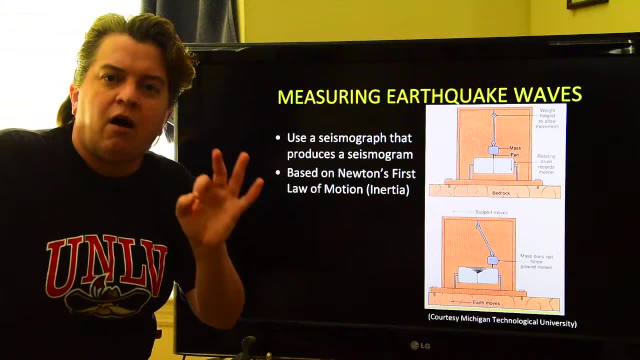 Well, this seismograph makes the seismogram and it's based off Newton's first law of motion, which is inertia. Remember, in inertia, an object in motion tends to stay at motion. An object at rest tends to stay at rest. 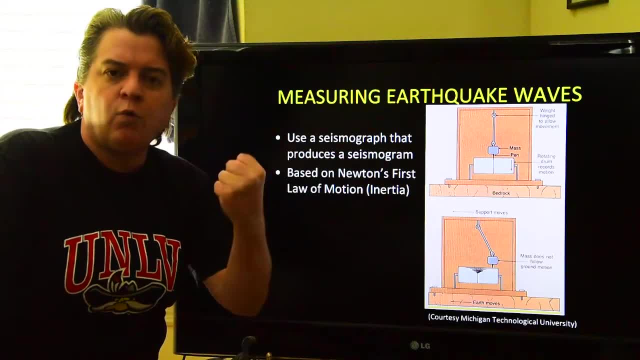 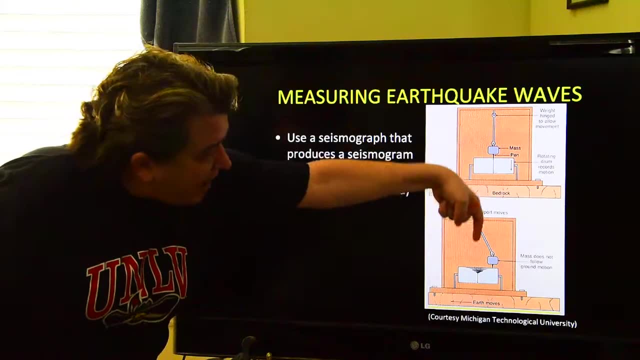 This mass in this pen is at rest, So it wants to stay at rest. But when the earthquake comes, the Earth moves right, And this is hanging right here And this Earth is moving underneath it. And so as the Earth moves underneath it, 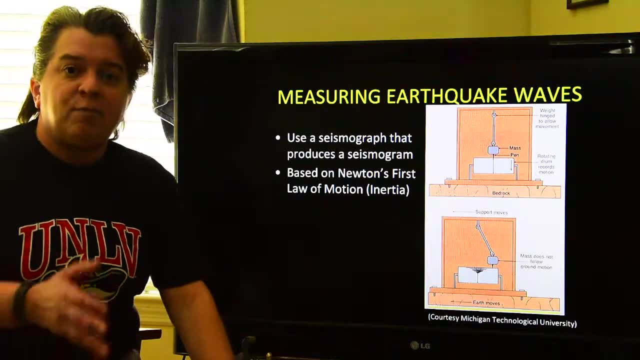 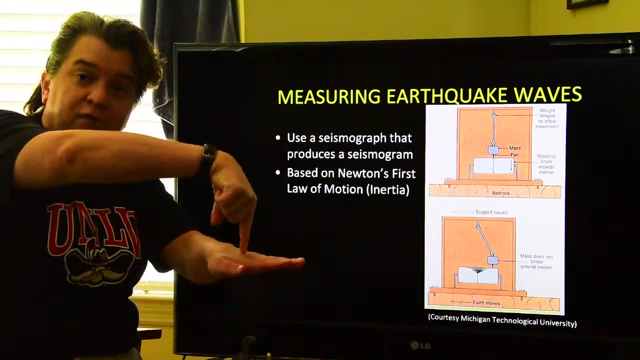 the squiggly lines are created, And that's basically how one of these works. Now, of course, Earth is three-dimensional, so it's not as easy as just having this pen sitting here like this. There's actually three of them.